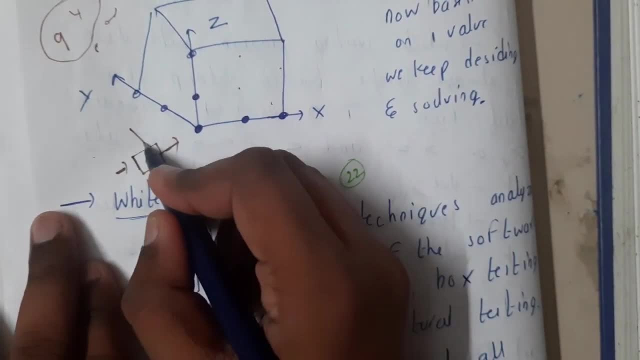 input and we know what we are getting as the output and we know the requirements, Whereas we don't know what is inside the logic or any kind of implementation or flow or anything right. So that is nothing but black box testing, black box testing, So, whereas in white box testing, 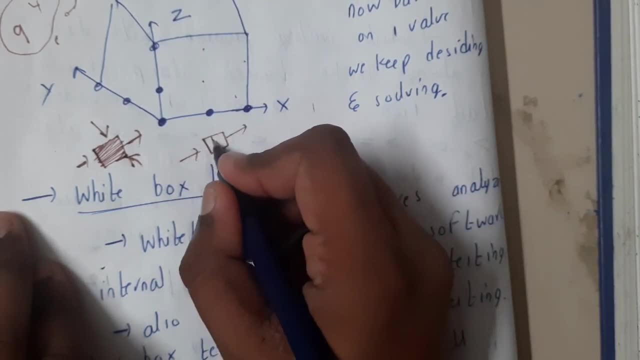 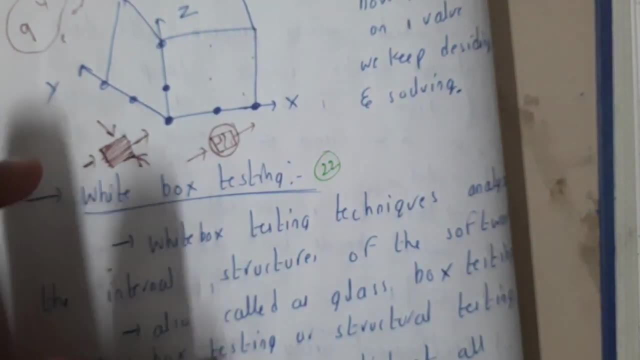 it is transparent, guys. you can say where you can see the, all the mechanisms or all the flow, or how the architecture is designed. everything you can see from the outside itself. So you can understand the logic behind that, right? Okay, so white box testing technique analyzes the internal. 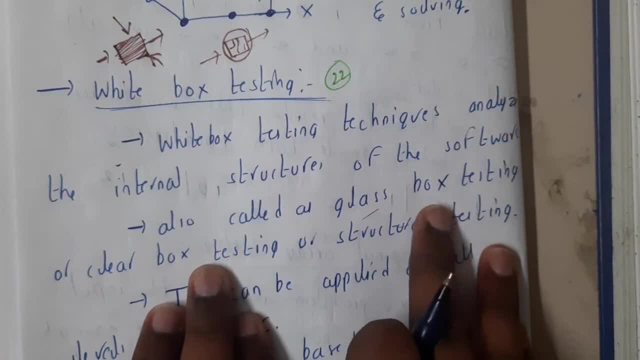 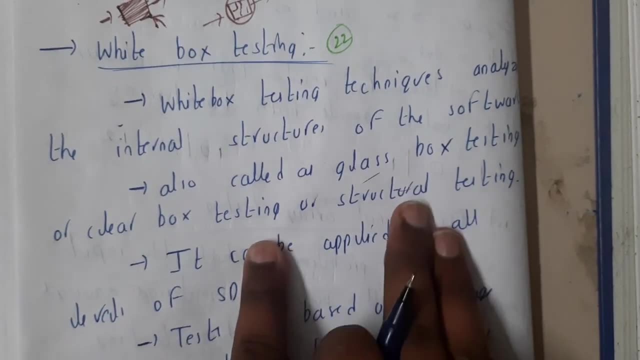 structure of the software. okay, Also called as a glass box testing guys. So it is transparent. So right, that's the reason why it is called as a glass box testing or clear box testing or structural testing guys. Okay, so it can be. 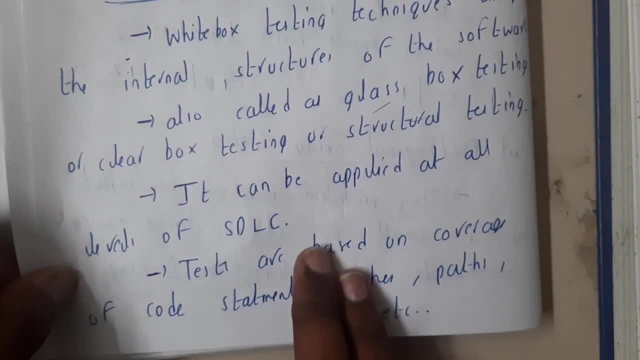 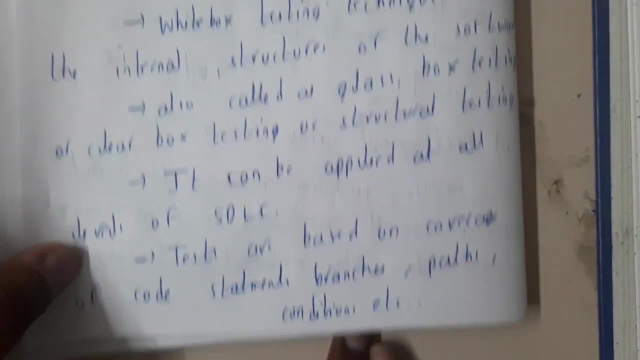 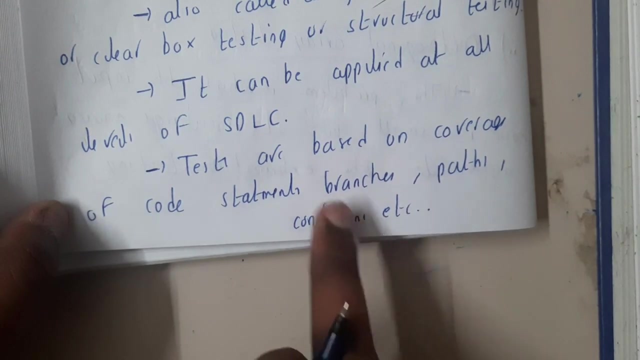 applied at any level or at every level of SDLC guys. So basically you will be writing the code and you will be testing right, So you can see that is also coming under the white box testing Okay, tests are based on the coverage of code statements, branches, paths and conditions, Guys. 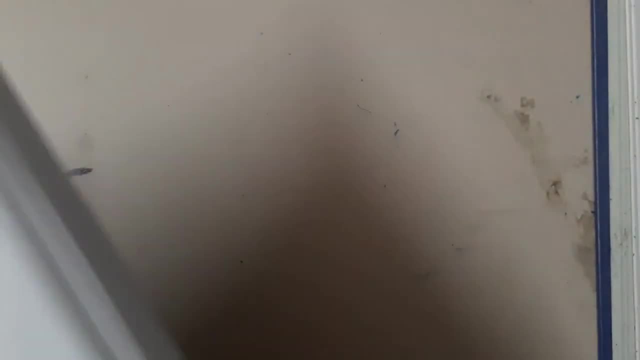 you will be understanding that, So you can see that, So you can see that, So you can see that, So you okay. so the more you understand it, the more you can understand it. So that's the reason why we are discussing about these things in detail now. only don't worry. Okay, so you can see the mechanism. 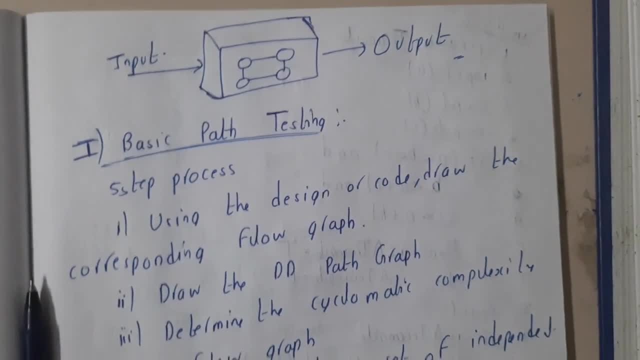 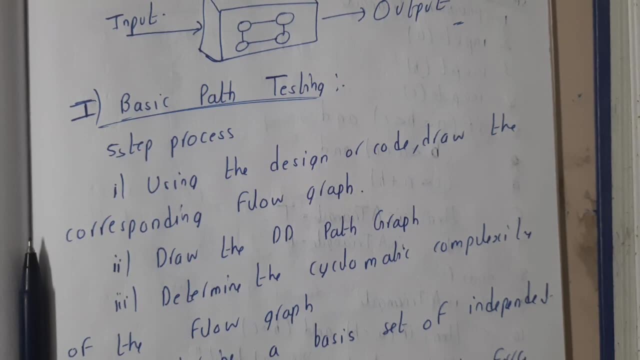 that water is the flow and how the architecture had design or how the components are connected. Okay, so now let us go through some basic path testing. So once we are done with this basic path will be going through controlled flow graphs, guys. Okay. so don't worry, it will. 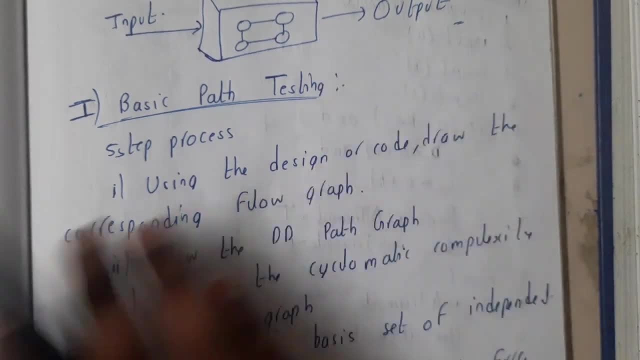 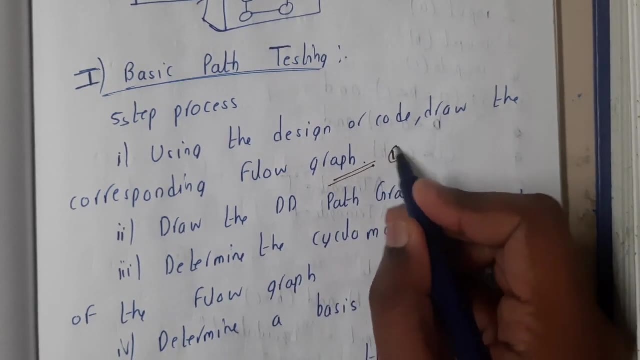 be hundred percent clear for you. Okay so, basically, in basic path testing, we will be having 5 Different steps, guys. Okay so, using the design or code, draw the model knowing theently underneath the monitor, Empty the corresponding flow graphs. so first thing that you will be doing is nothing, but you will be. 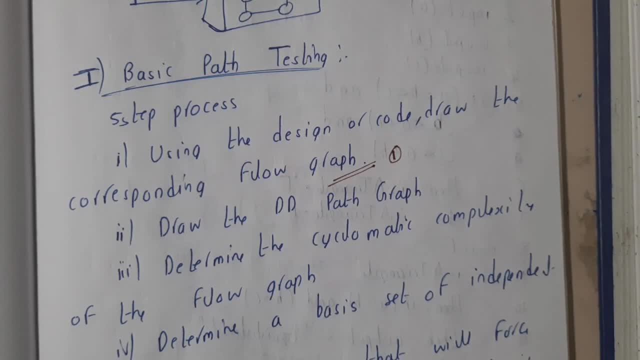 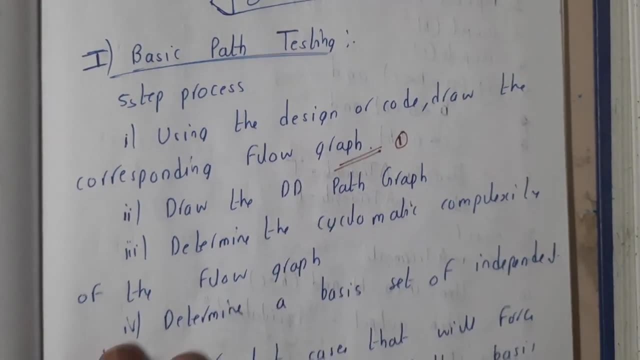 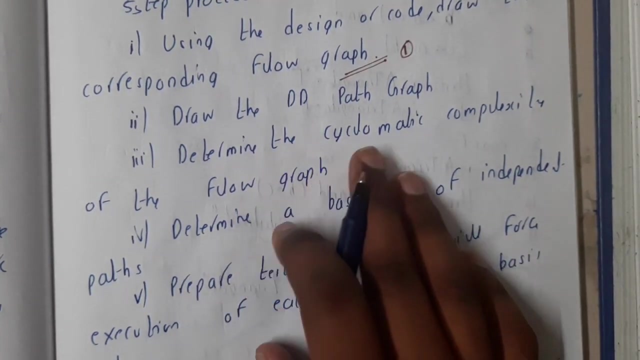 drawing a flow graph. so, once you have drawn the flow graph, you will be marking the dd path graphs, guys. so what are all the possible paths in which you can travel? so you'll be drawing them all and then you'll be determining the sorry you. you will be determining the cyclometric complexity of. 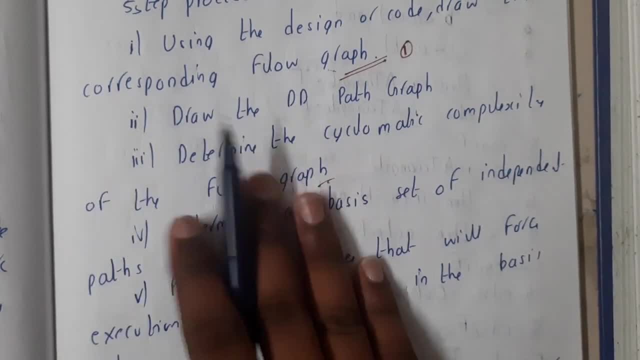 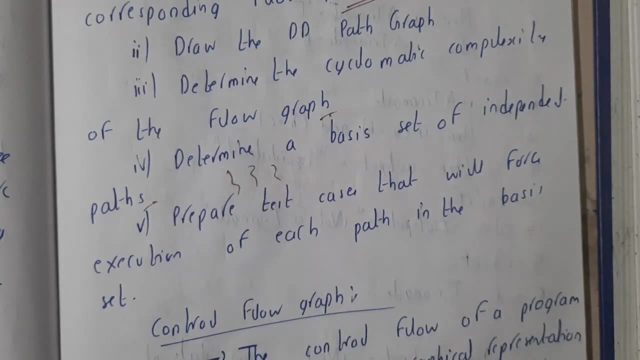 the flow graph. okay, guys, we'll be discussing about these five steps now, only don't worry. okay, so then you'll be determining a basic set of independent paths, like what are the different different paths you can follow, and at the end you will be preparing the test cases that will focus. 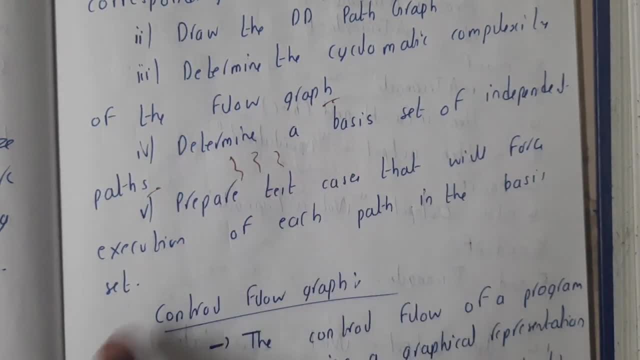 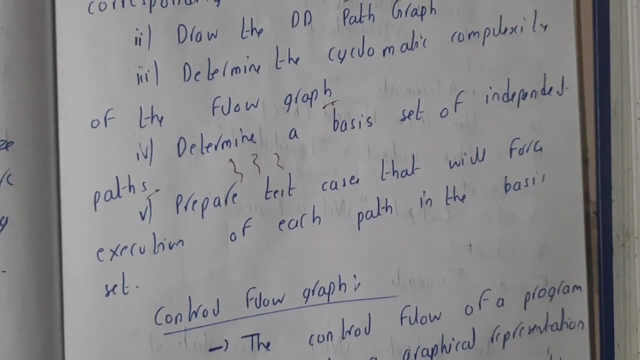 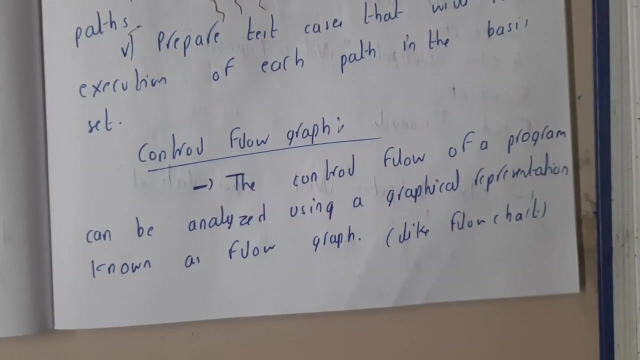 and executing of the each and every path of the basic set. okay, so this is just of the five steps. guys, we'll be discussing about these five steps now. okay, so i told you the first step is nothing, but you need to draw a flow graph. okay, so the flow graph, or the control flow graph in detail: 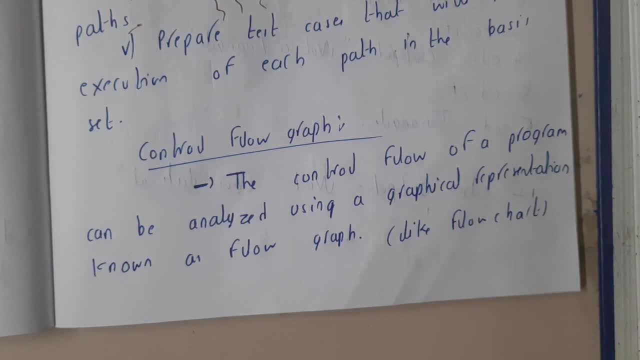 you can say it is as a control flow graph. okay, so the flow graph or the control flow graph in detail. you can say it is as a control flow graph because it is saying about the control flow, how the controls are flowing from one step to another step. okay, so the control flow graph of a program can be analyzed using a graphical structure known. 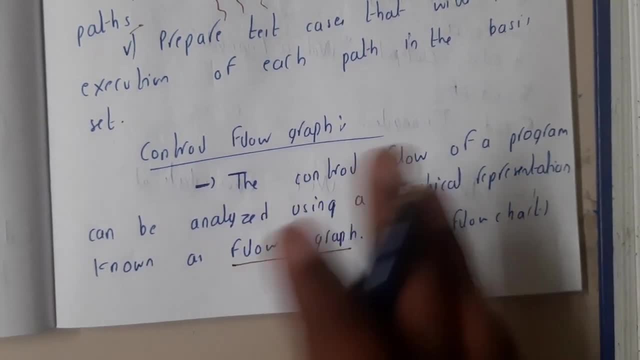 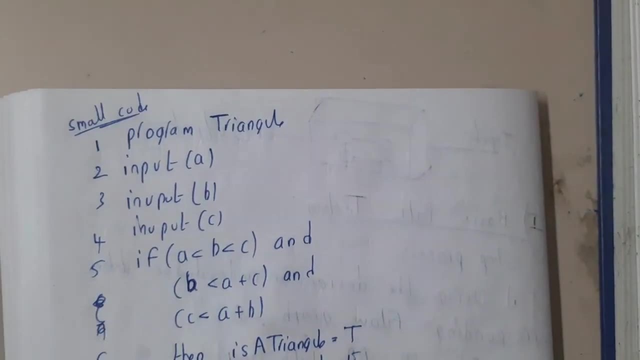 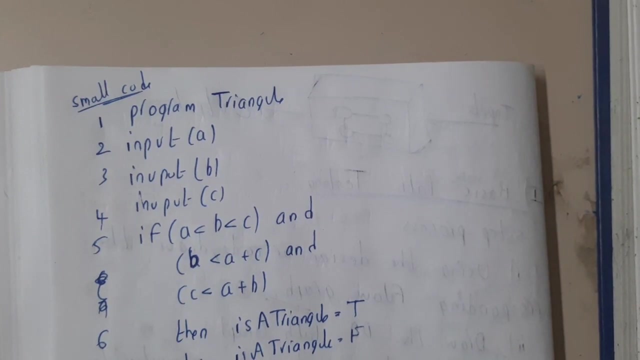 as flow check, flow graph. so it exactly looks like a flow chart, guys, okay, okay. so first let us go through an example, and for this example we'll be developing the whole thing, guys. so for this only, we'll be continuing the all the five steps, okay, okay. so here we are writing a code for the flow. 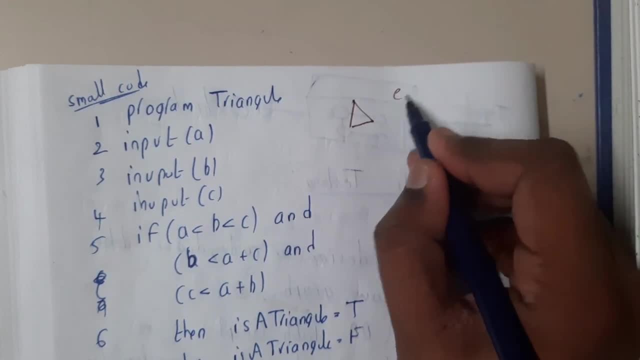 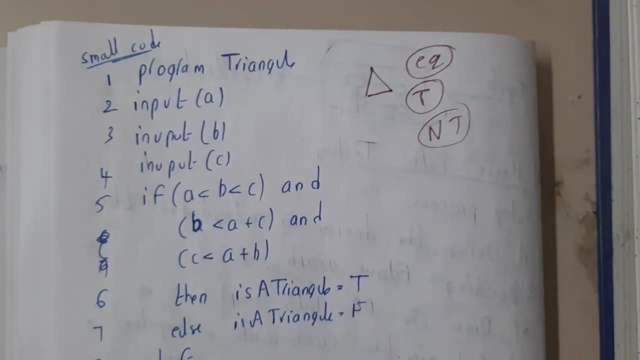 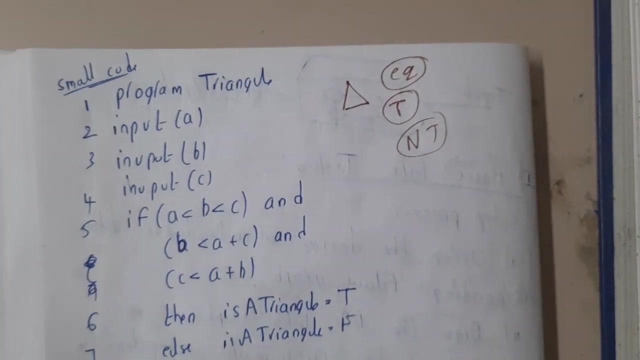 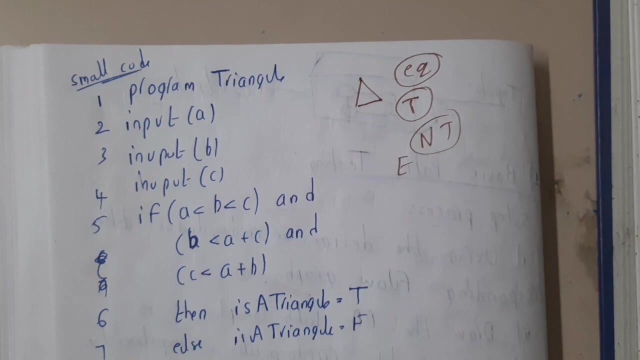 graph and here we will be stating that whether it is an equilateral triangle or a normal triangle or not, a triangle, okay, and which is not an equilateral triangle, also okay. so, basically, you will be saying that whether it is equivalent or equilateral triangle or not, equivalent triangle, okay, okay. so now let us go through the theoretical parts, guys. 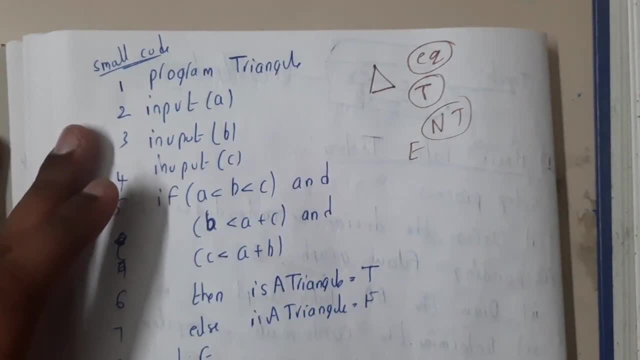 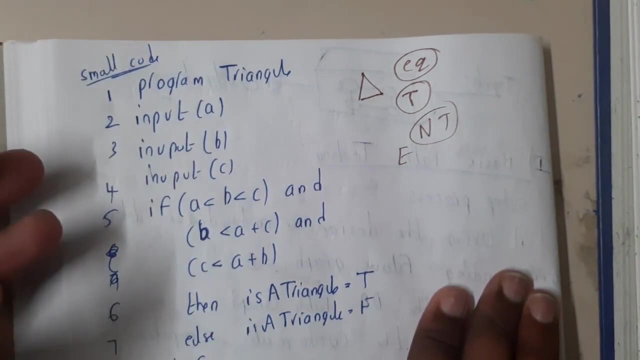 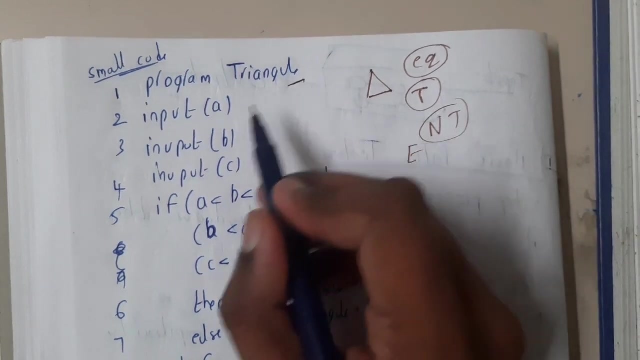 okay, sorry. so the code will be in this way, guys. so let us assume you are writing the code in python or any kind of language like ruby also, you can assume, guys, because this syntax is almost nearer to python and ruby. okay, so initially you will be starting the program triangle, so you will be. 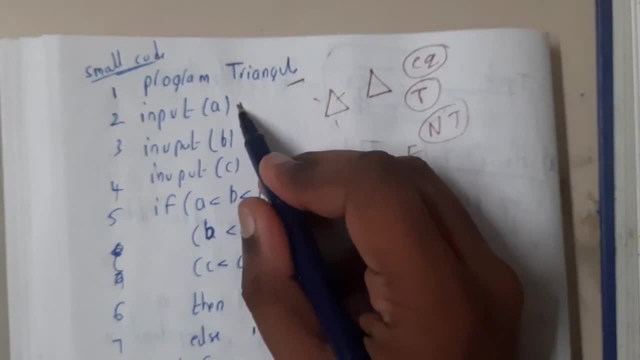 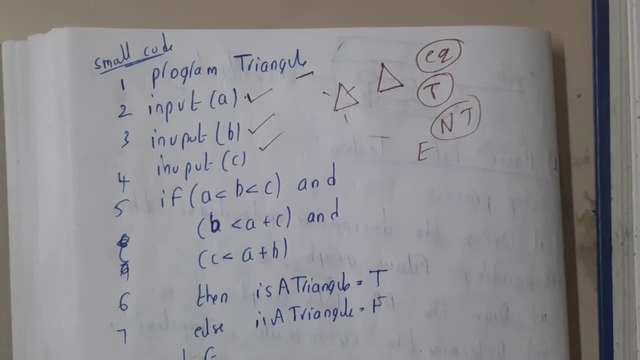 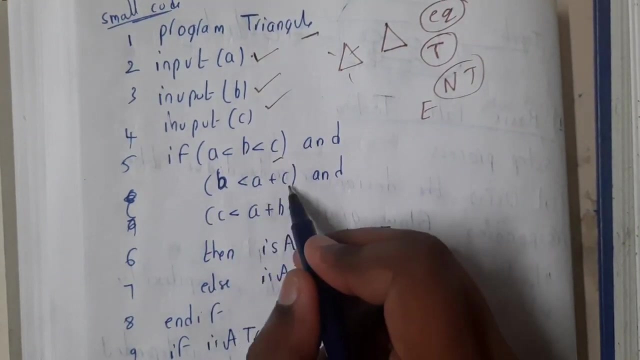 taking the inputs. so triangle will be having three sides, so you'll be taking the inputs a, b and c. okay, so the first thing that you should remember is the condition for a triangle, guys. okay, so a should be less than b, should be less than c, and b is less than a plus b and c is less than. 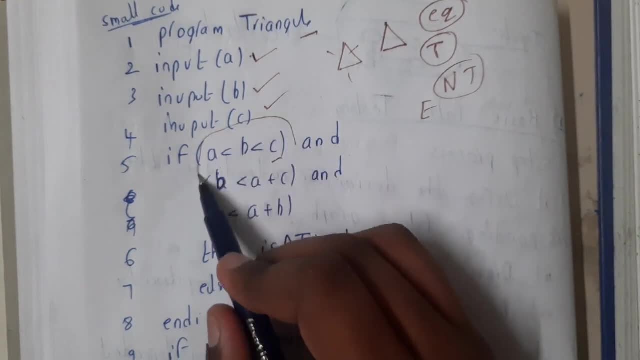 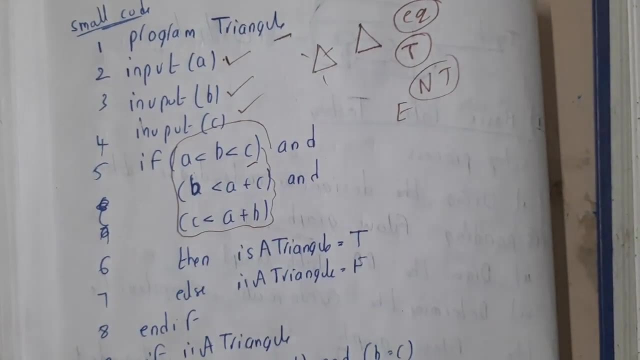 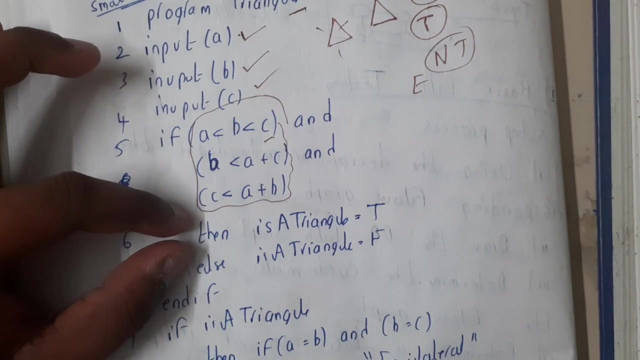 a plus b. so this is a common condition which any proper triangle will be following, guys, so any kind of triangle you design. so just to take some examples, you can understand guys, okay, okay, so if everything is passed, then you can assume that that has a triangle, guys. 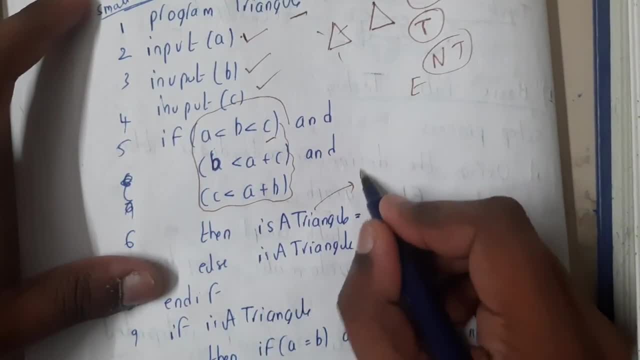 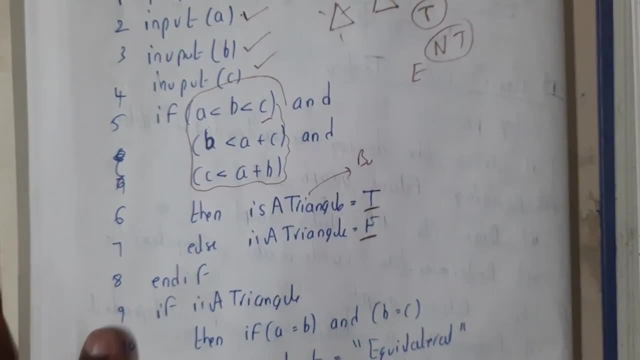 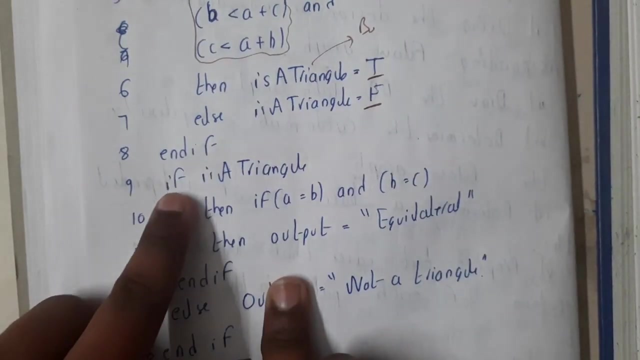 okay, so here i am using is a triangle, is a boolean guys, so i'll be storing true inside it. else, if this is false, i'll be directly storing the false in it. f okay, so now we are ending this. if else, if sorry, if statements so end. if so, after that you are starting another. if so, based on the. 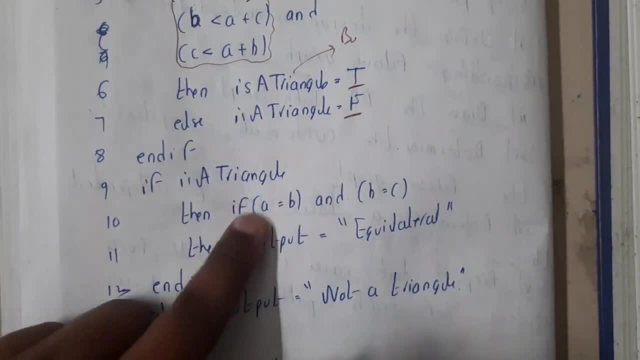 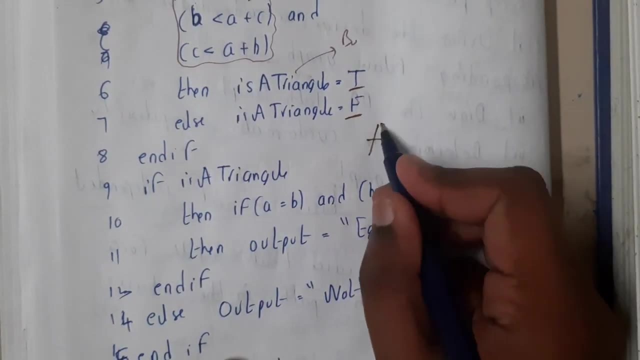 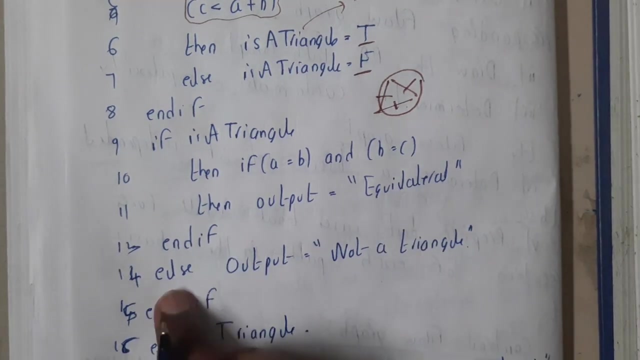 output that you got. so if e is a triangle, if it is a triangle, then if a is equals to b and b is equals to c, so if a is equals to b and b is equals to c, then indirectly it's an equilateral triangle, and if else output is equals to not a triangle. okay, so here we wrote this part so, but i forgot. 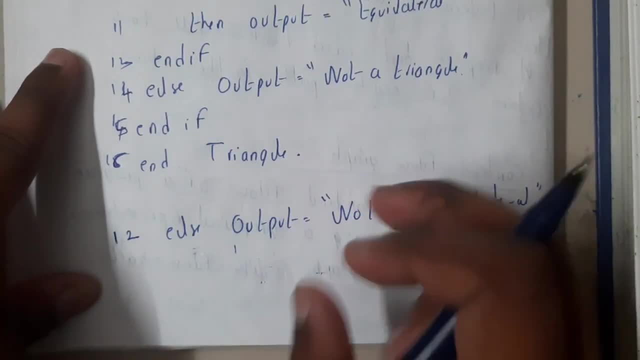 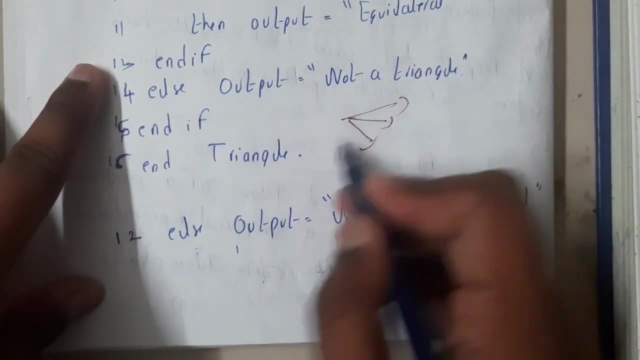 to write about the not, not equilateral triangle, right? so a triangle can be equilateral or not equilateral, right or not a complete triangle. so we are having three different outputs here. okay, so at line 2l you will be writing else, output equal to not equivalent. so then you will. 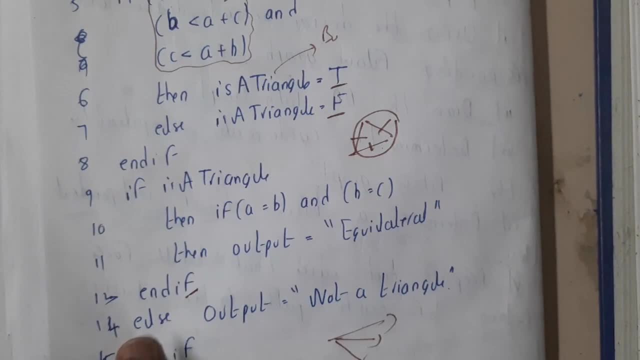 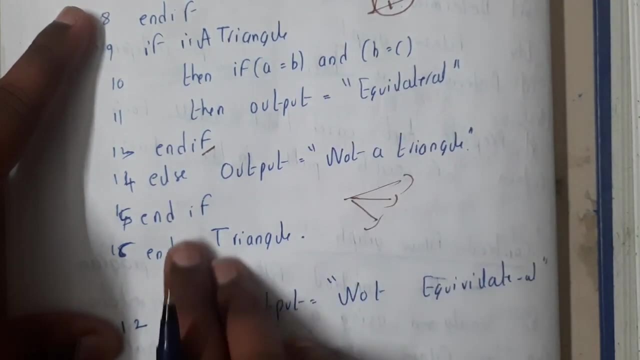 equilateral. so after that you will be ending that if and the else of this part of this. if you'll be here, if output else output equal to not a triangle- okay, so then you'll be ending if and you'll be ending the triangle function, okay. so i hope everyone got some basic idea right. so we are. 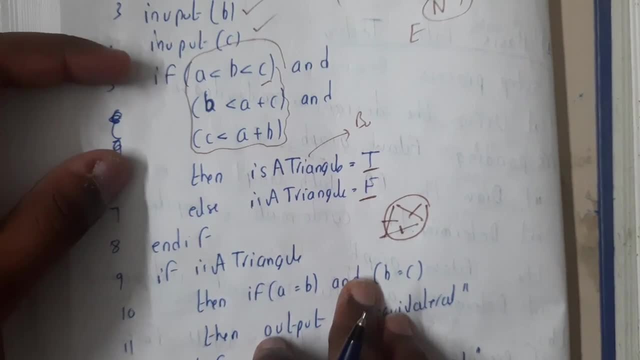 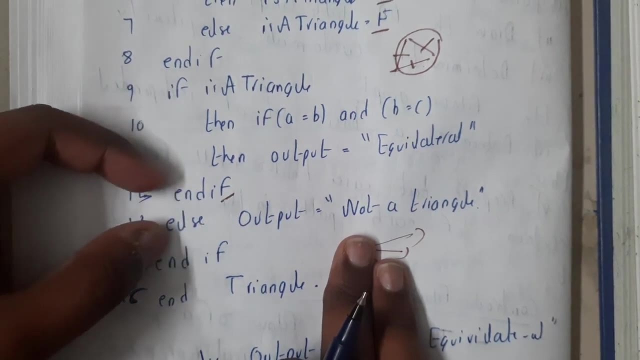 having totally two decision makings, guys. so here we are making a decision whether it is a triangle or not, and here we are making a decision that is nothing but whether it is an equilateral triangle or not. equilateral triangle, simple, okay. so if you draw the flow chart, it will be in this way, guys. 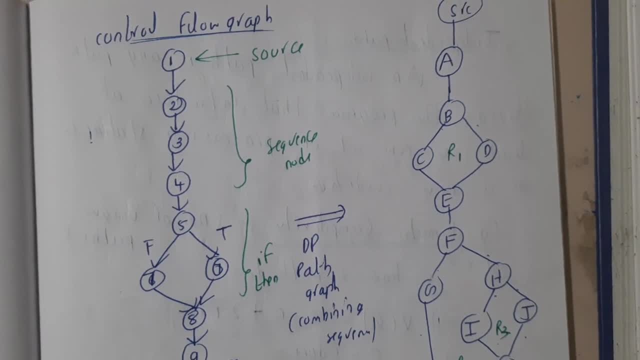 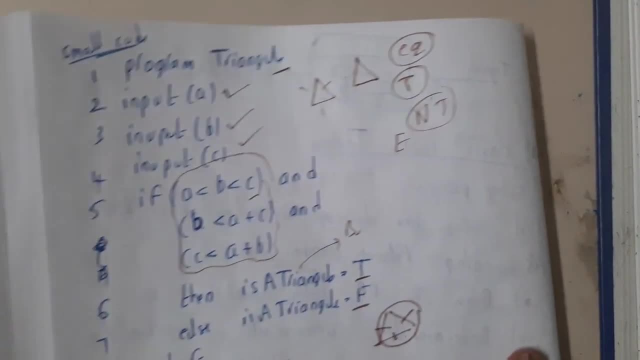 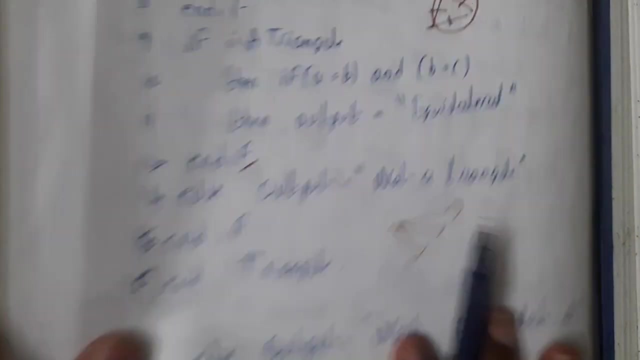 okay, okay. so the first step is nothing but the program. so, if possible, please take a paper and write down this code, guys, because while explaining the flow chart, it will be clear for you. so i did mention the line numbers also, so that we can just point out them in the graph. so the first step, guys, i'll 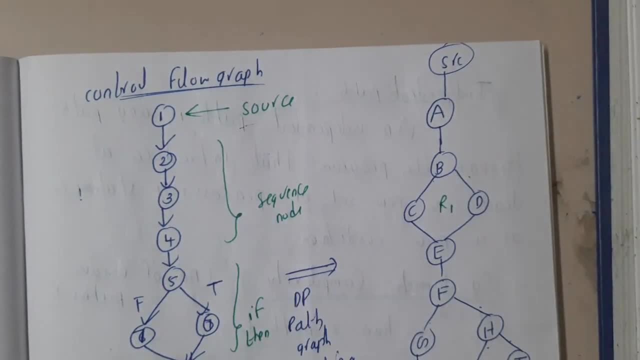 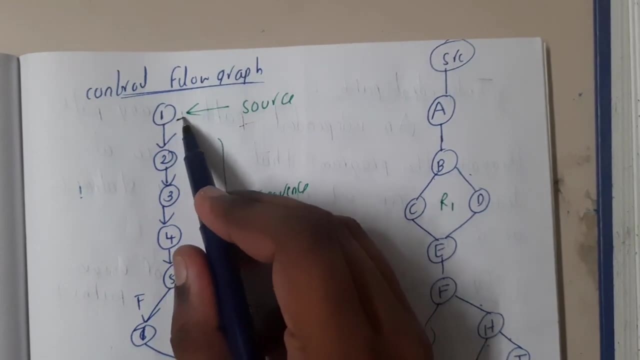 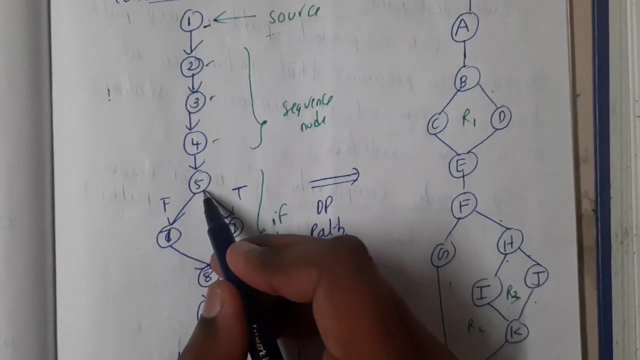 be observing on the left side because it's on the program is on the left side, so i'll be reading it and we'll be understanding what we have drawn in this flow graph. okay, so the first step is nothing, three steps are nothing, but we took inputs, so after that is our decision, guys. so if it is true, 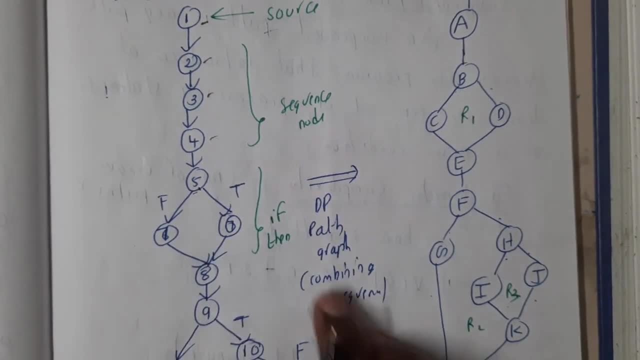 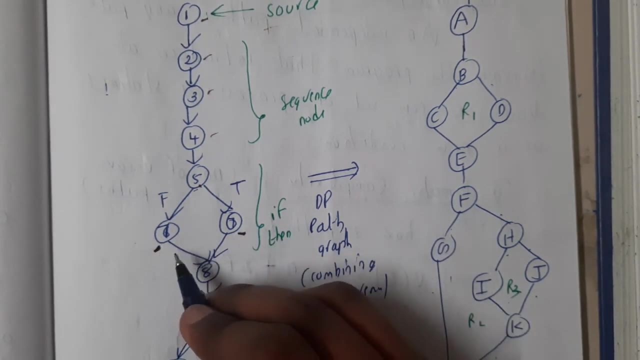 we'll be going one direction. if it is false, we'll be going another direction. so if it is true, we will be saying that it is a triangle. if it is not true, we'll be thinking that it is not a triangle. okay, guys, here we will not be printing anything, so please remember that. okay, so once it is done, then 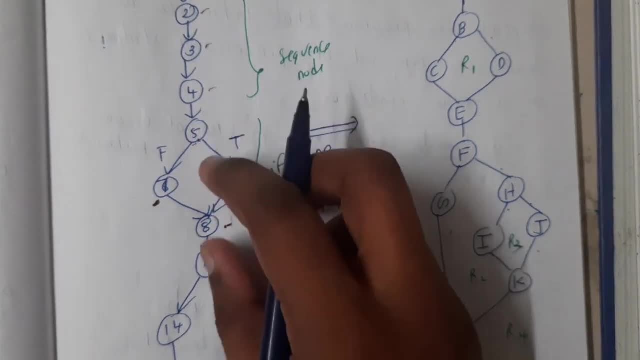 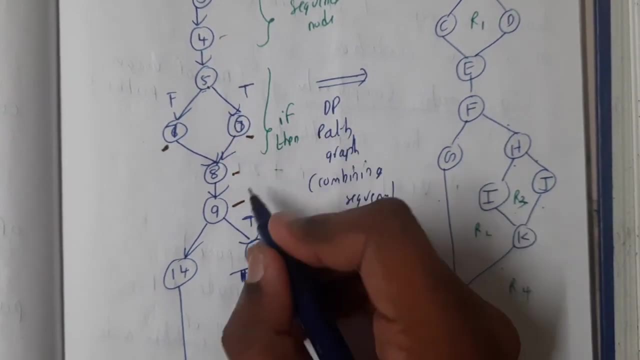 you will be connecting to end, if you will be closing this, if else, if statement and then you will be moving on to your next decision. so here you will be checking whether it is true or not, whether the output that you got here it is a triangle or not. if it is a triangle, you will be. 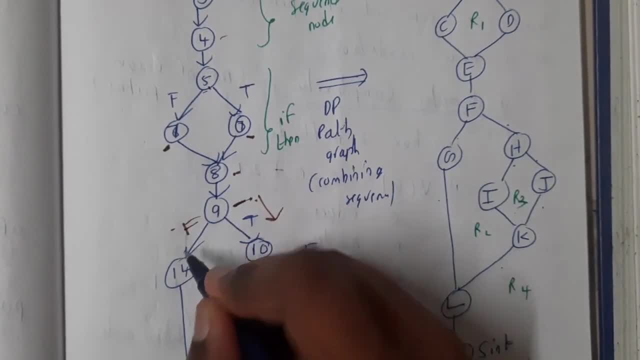 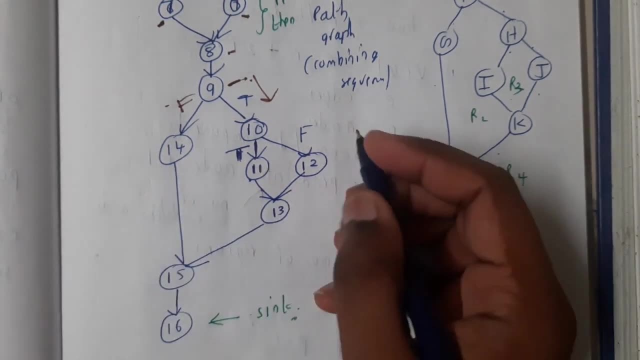 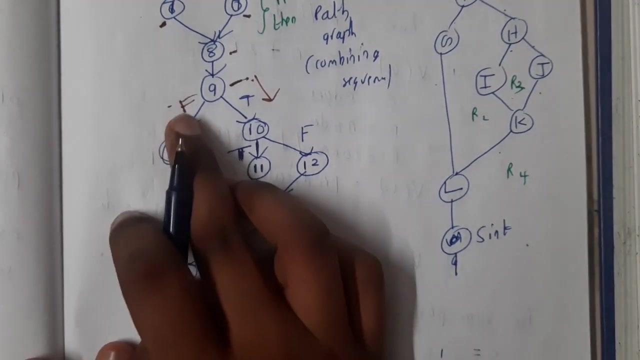 moving to this side. if it is not a triangle, you will be moving this side. so if it is not a triangle, you will be directly printing that it is not a triangle, right? so that is nothing but the step here. okay, okay, so i think. okay, that's what it is. 14, right? sorry, i was just a bit confused, okay, so. 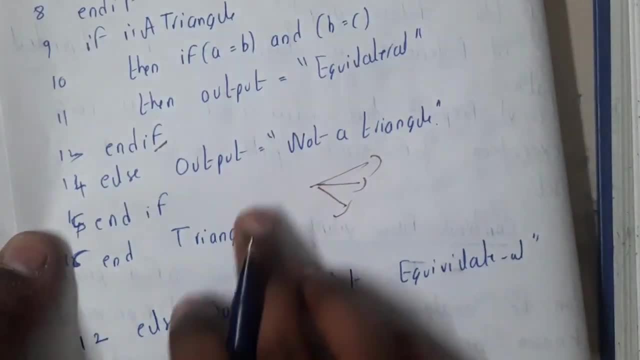 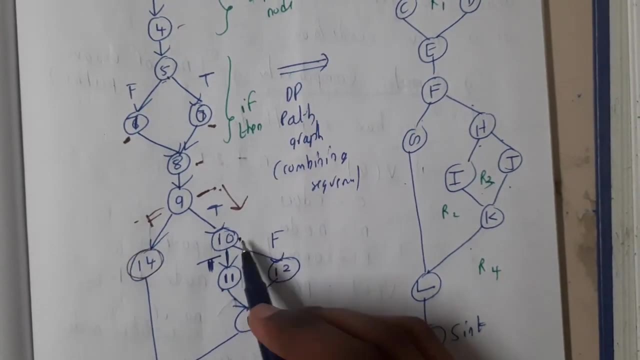 if it is false, you'll be directly printing the 14th statement. 14th statement is nothing, but it is not a triangle, okay, okay. so, similarly, if it is true, you will be going through 10th. 10th is nothing, but it will be checking whether. 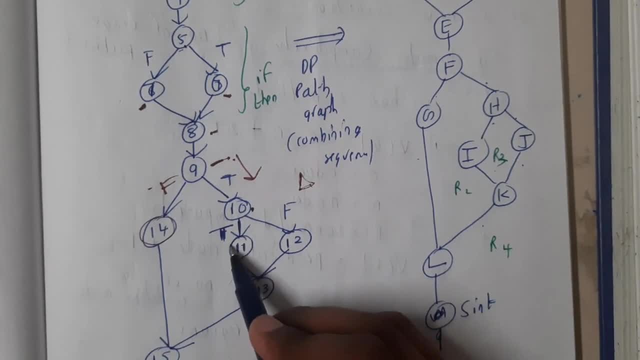 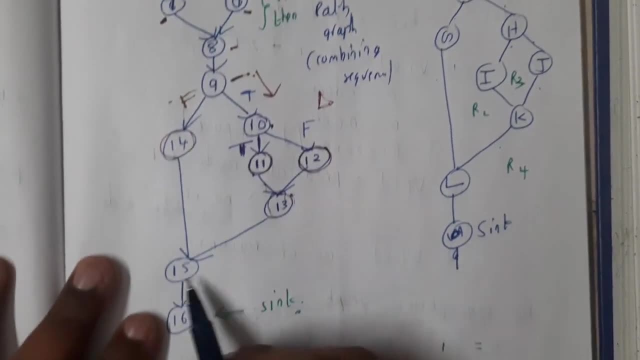 the triangle is equal, equilateral or not. so if equilateral, you'll be printing is equilateral, if it is not equilateral, you will be printing not equilateral. so once it is done, you'll be closing the if and after that you'll be going through 15. that is nothing but end of the. 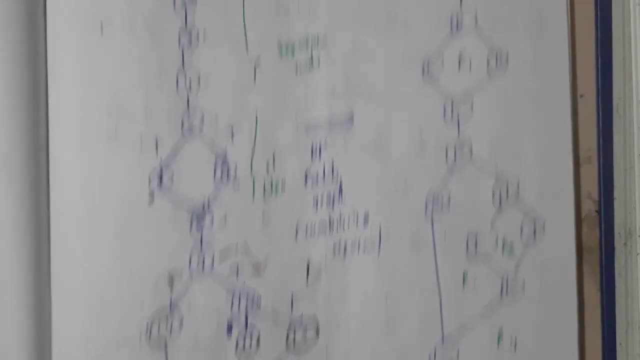 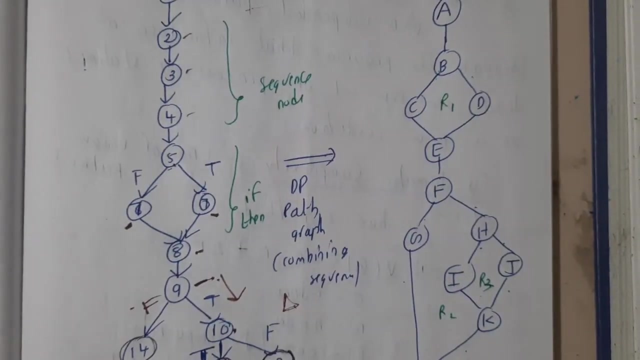 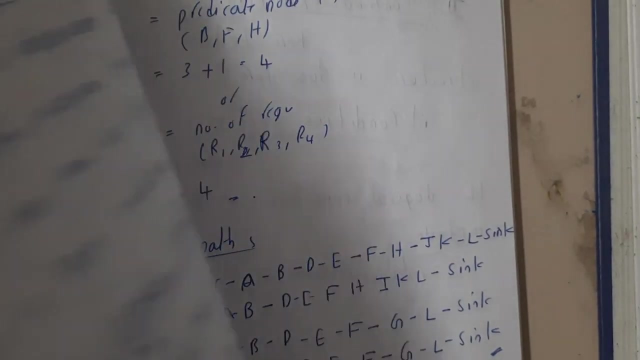 triangle. okay, so this is nothing but sink. so basically, we have added one source and one sink, guys, at the end. okay, so source is the starting and sink is the ending. okay, so now let us convert this flow graph into a dd path graph, guys. i did inform you about a dd path graph, right? so dd path graph is. 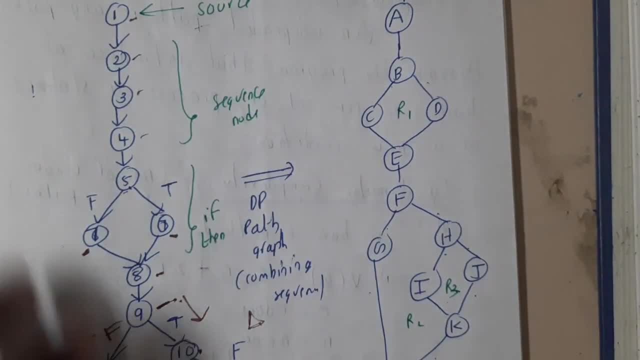 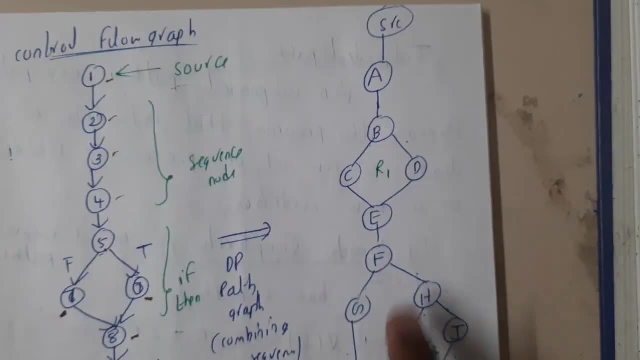 nothing but a simple version of this whole graph. so here, if you observe, here we are having sources, so write one source and we are having one sink, you'll be writing one sink, okay, so after that we are having here a sequence of steps, right, so combine them all and assume them as a guys. simple. 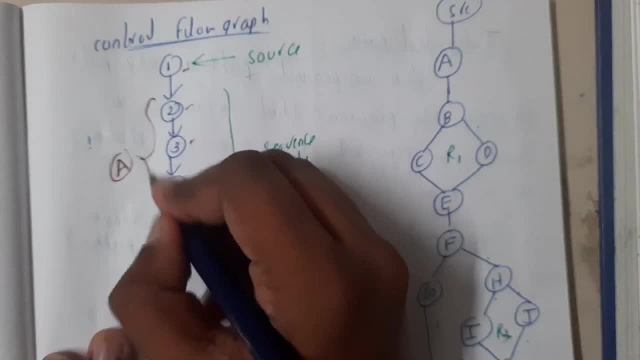 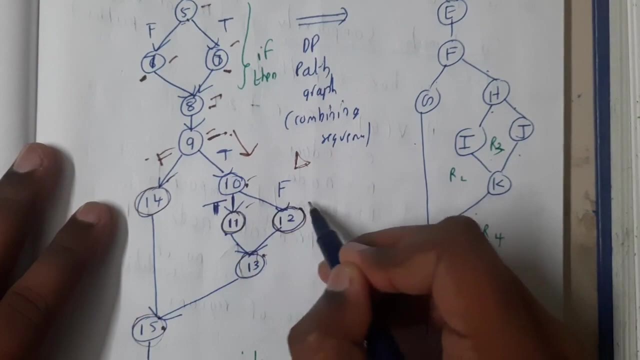 right, so i'll be writing them here, so assume them as a after combining them. so we got a and this is c, this is d, this is e, f, g, h, i, j, k, l, m. that is nothing but sink, so in this way you will be naming it. 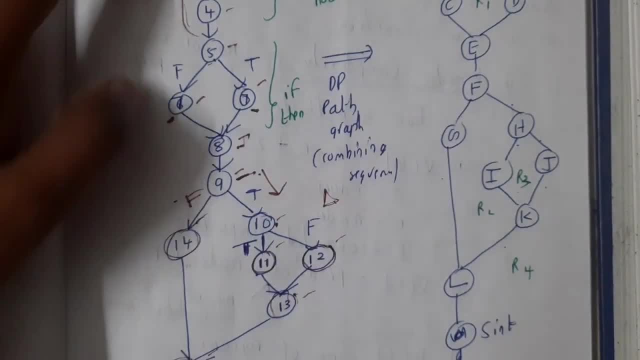 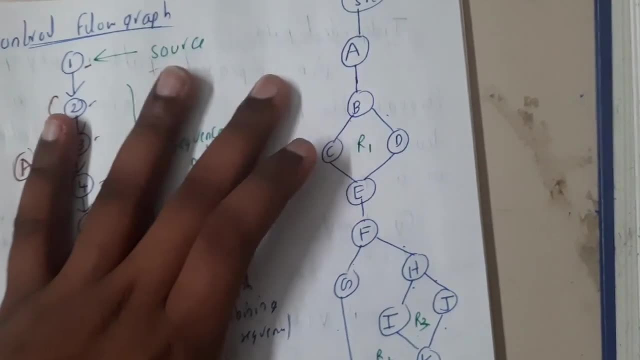 guys. so, basically, here there are a sequence of steps, whereas else, anywhere, we are not having any kind of combinations to combine things, guys. so that is the reason why we combined all of them and we made a simple dd path graph, okay, okay. so now, if you recall the second, the next step we need, 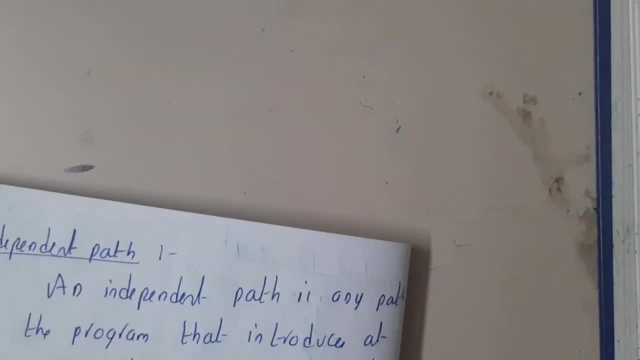 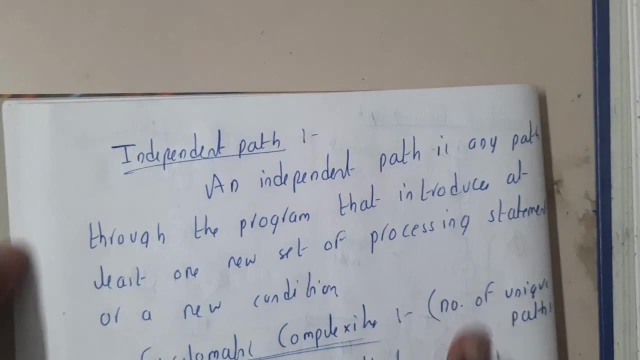 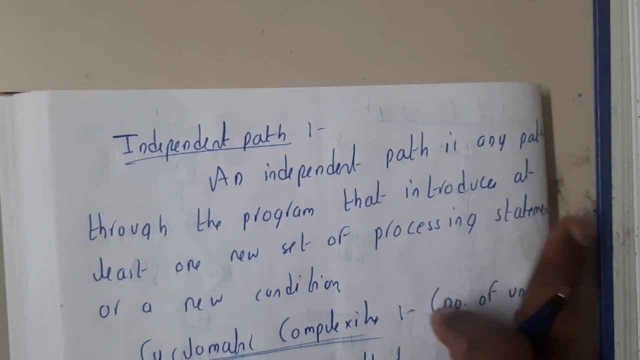 to calculate a, calculate a number, or that is nothing but cyclometric complexity. so before going to that, let us go through some basic definition. that is nothing but independent path. okay, so basically, an independent path is any path through the program that introduces at least one new set of processing statements. 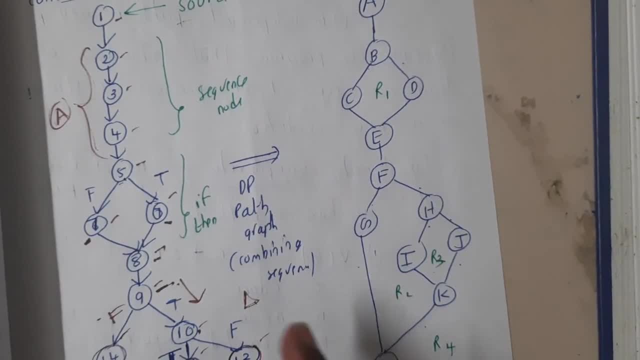 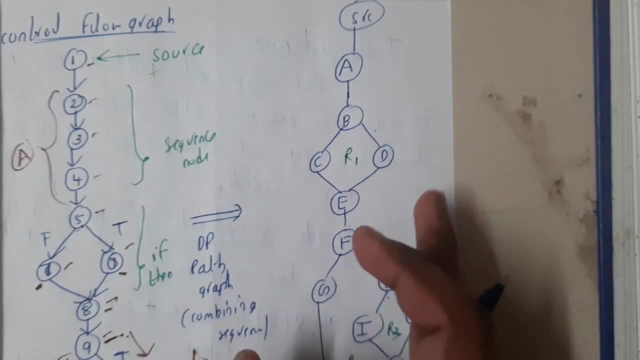 so if you ask me in this flow graph or dd graph graph, how many paths are there, you might be asking me. so just observe me, guys. you guys will be discussing about this again, so don't worry. so initially you'll be starting at source and let us go through the left part first. 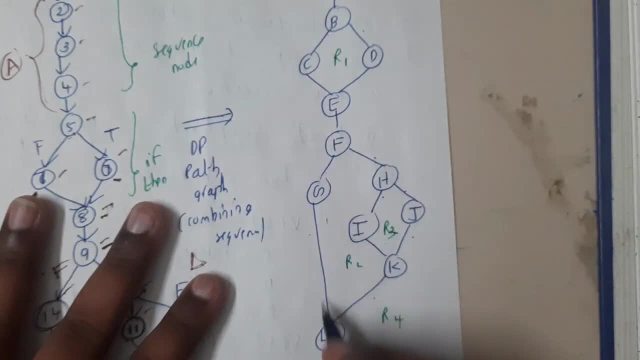 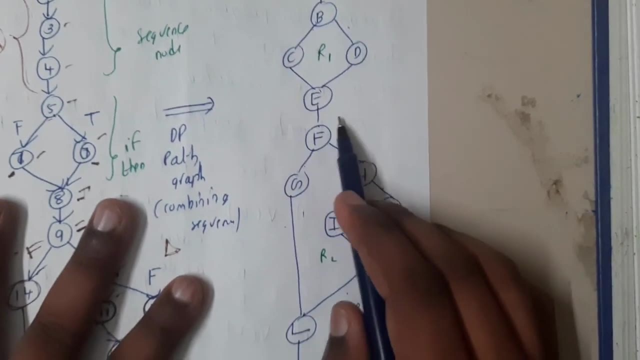 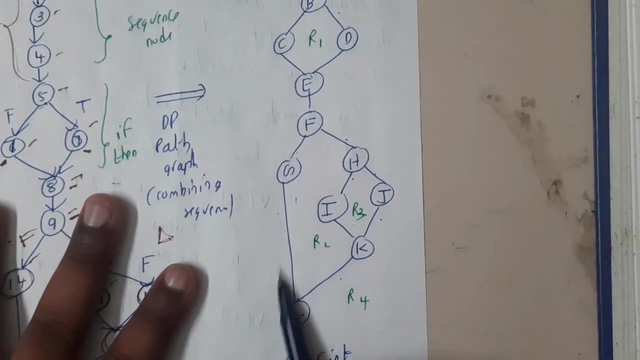 so you'll be going like this: you've traversed, so that is the first path, the second path, second path, similarly the third path. okay, so these are the three main paths, guys. after that we can go from this side also, okay, so in that way you will be having multiple paths. you can say: okay. 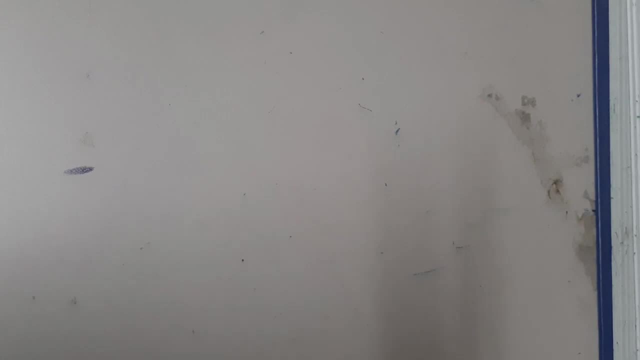 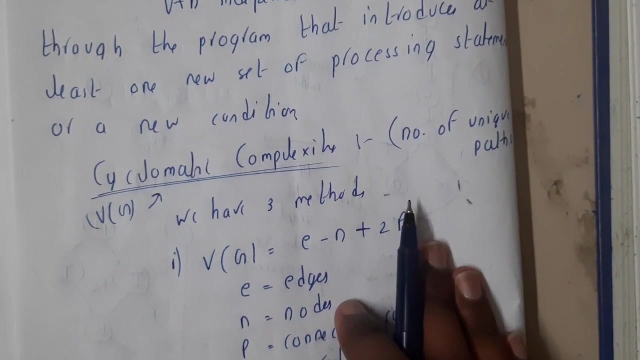 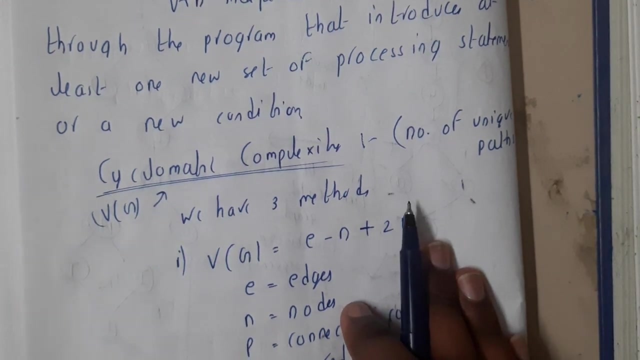 okay, okay, okay, okay. so now let us continue. okay, so now let us calculate the psychometric number. that is nothing, but we are having three different formulas, guys, you can apply any one or you can just recheck with applying every formula. okay, it is quite simple. so here we have three methods. that is nothing, but v of g is equals to: 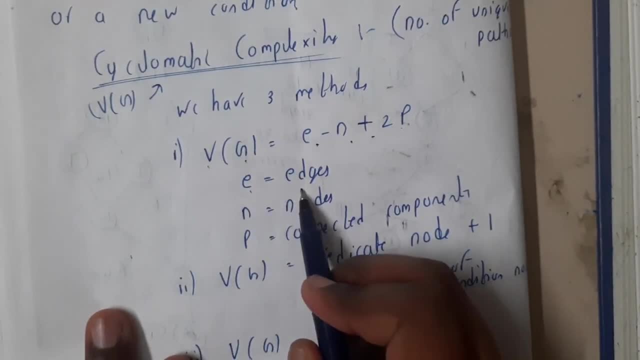 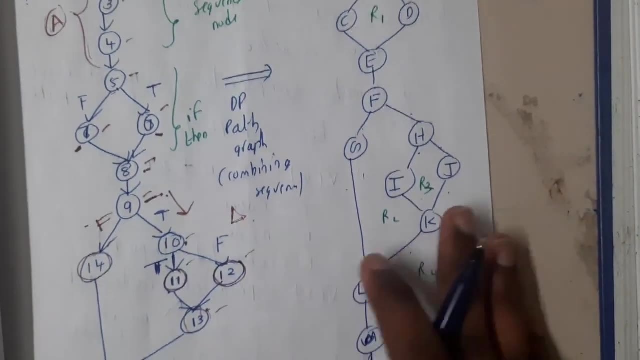 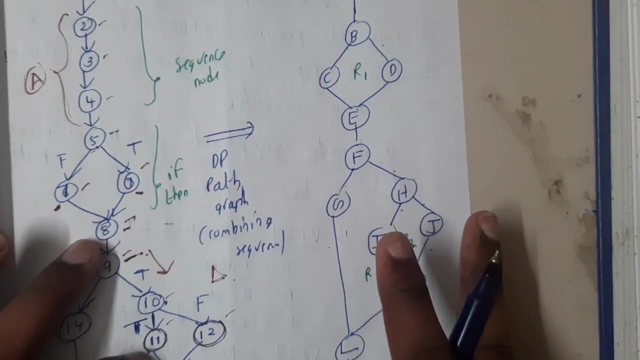 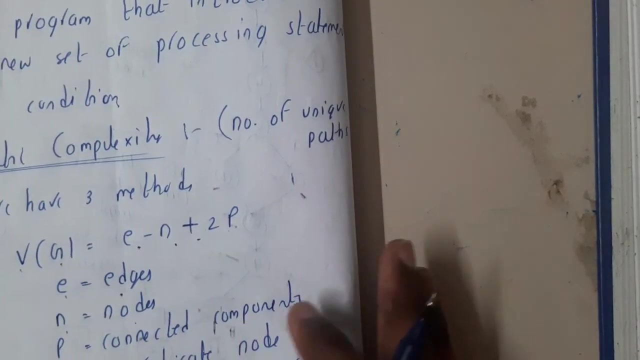 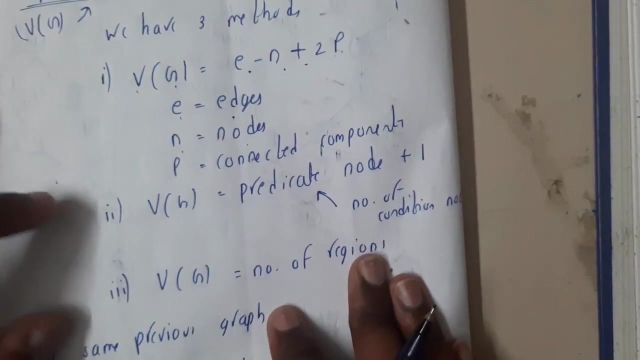 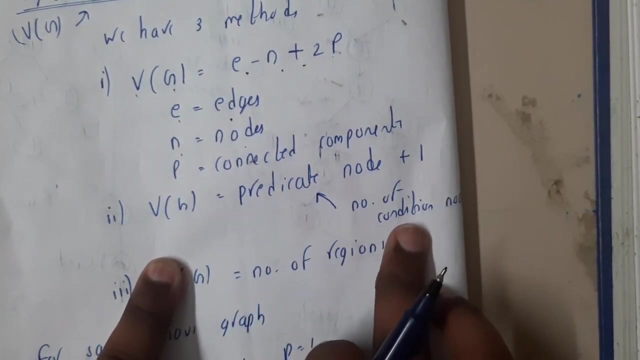 e minus n, my n plus 2p, that is nothing but e indicates the edges, n indicates the nodes and p indicates connected components. okay, say, if you count- sorry, if you count the components for this graph, you will be getting 16 edges, 14 nodes and two connected components. okay, okay. so once you get those things, you'll be just okay. sorry, you'll be getting only one connected component, guys. okay, okay. so once you got that, you will be calculating it. so, similarly, we are having a v of g is equals to predicate a node plus one. that is nothing but number of conditions. we are having three conditions, right. so similarly, we are having a v of g is equals to predicate a node plus one. that is nothing but number of conditions. we are having three conditions, right. so similarly, we are having a v of g is equals to predicate a node plus one. that is nothing but number of conditions. we are having three conditions, right. so similarly, we are having a v of g is equals to predicate a node plus one. that is nothing but number of conditions. we are having three conditions, right. so similarly, we are having a v of g is equals to predicate a node plus one. that is nothing but number of conditions. we are having three conditions right, so similarly we are having a. v of g is equals to predicate a node. 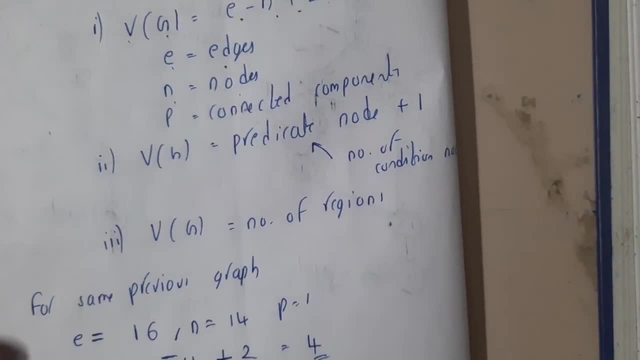 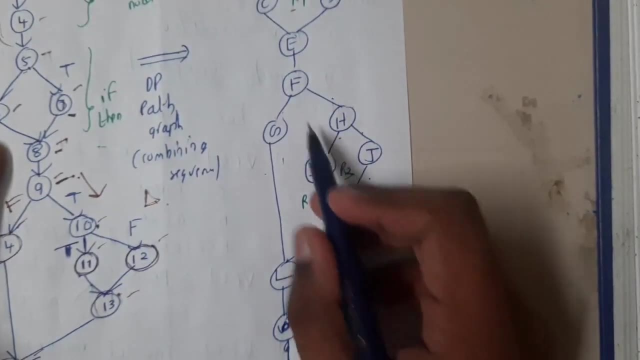 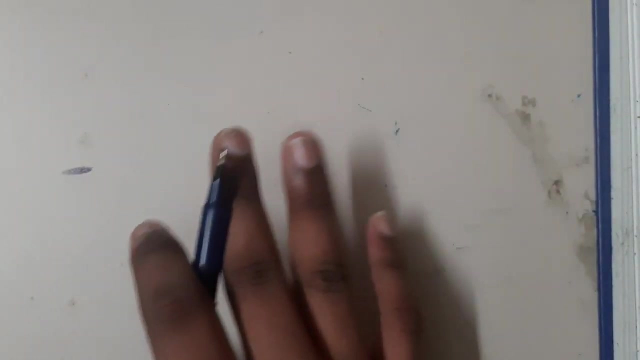 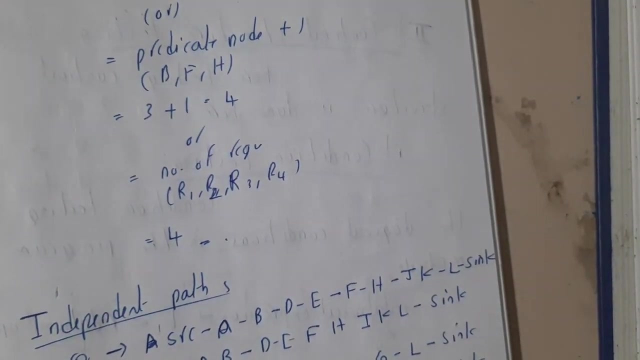 so three plus one. similarly, v of g is equals to number of regions also. so regions are nothing but a particular block. so here this is a locked region, right? so this is region one. here we are having- in this shape- that is region two, in this shape- region three and the exterior whole part is region four. so we are having four regions. so by using any of the formula you will be ending up with the result of four. okay, so now let us try to find the independent paths, guys, from source to sink. okay. 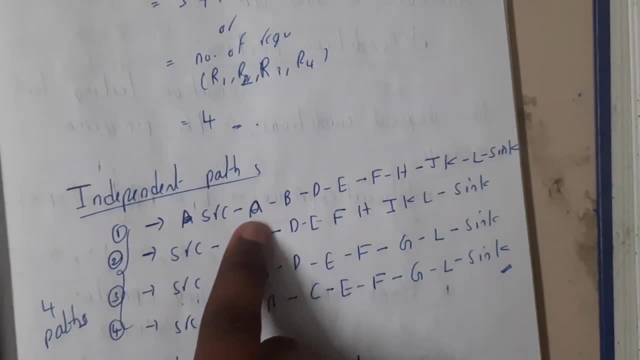 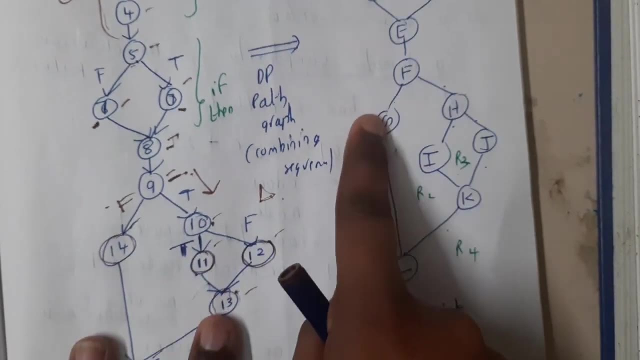 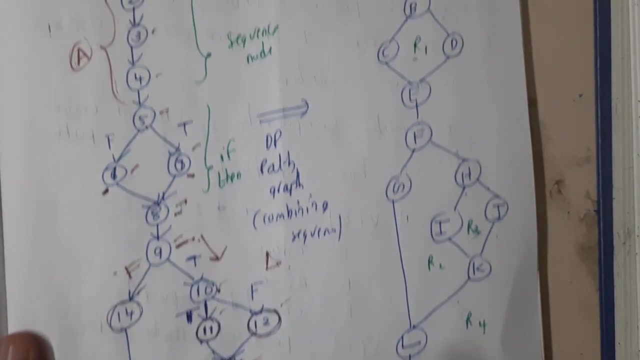 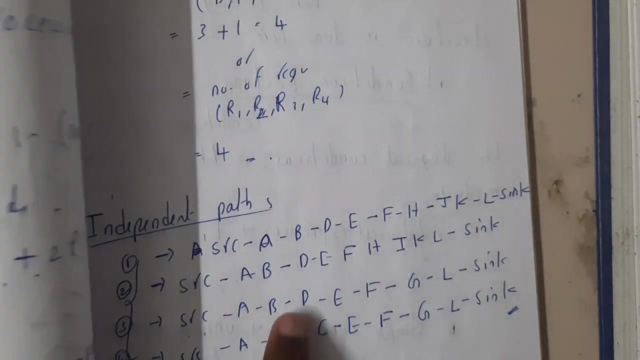 so the first path is from source to a to b to d to e. okay, so it is in this way. okay, so that will be our first path, guys. okay. similarly, the second path, okay. okay, just give me a second, guys. a, b d e. a, b d e, f h. okay. 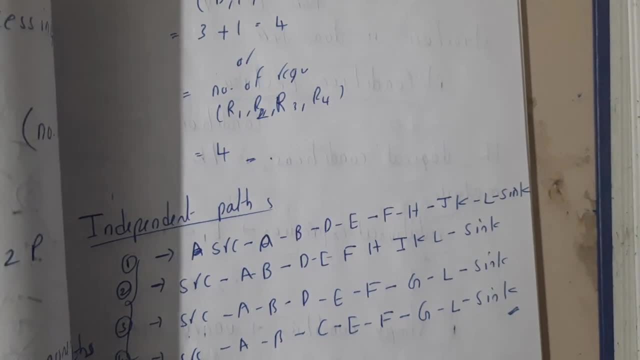 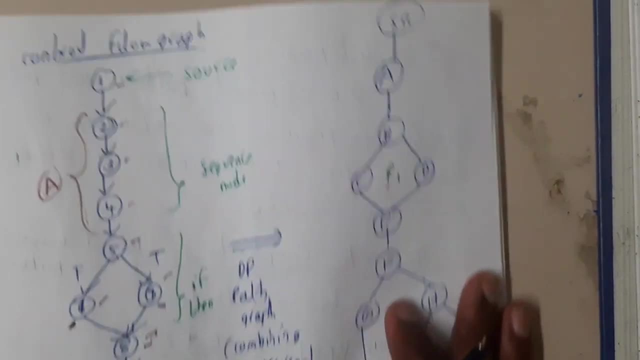 okay, just give me a second, guys, i'll be back in a moment. okay, sorry guys, i am back. okay, so basically there are particularly four paths in this graph, guys, okay, so here we are checking. so before going through the paths. so previously i told that we are having six paths, right, so i was. 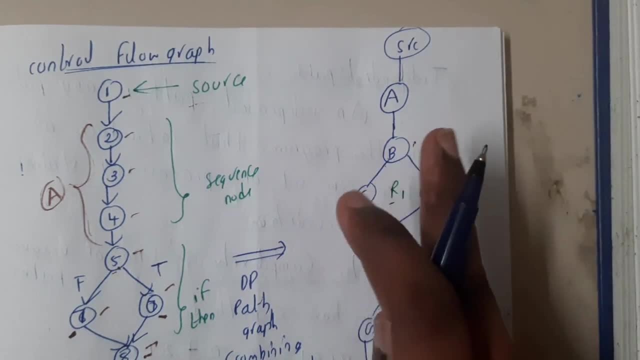 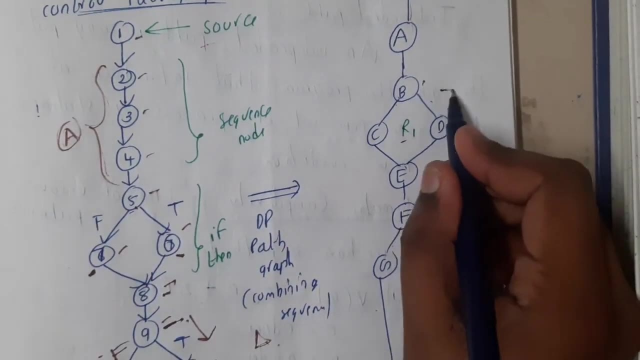 wrong. so basically there are only four paths, because the two paths which i thought were wrong, okay. so basically here we told that it is true, right, so from here on, you can observe. so here, if it is true, you will be going in this way. if it is false, you will be going in this way. if it is. 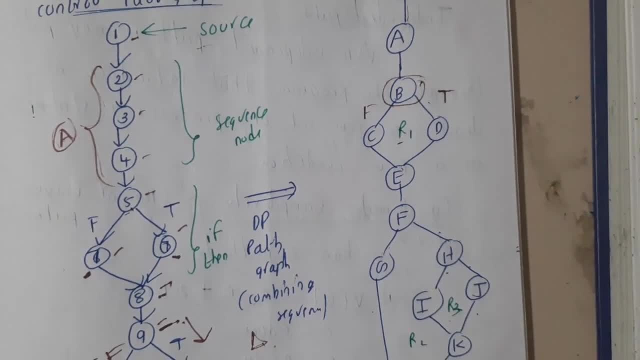 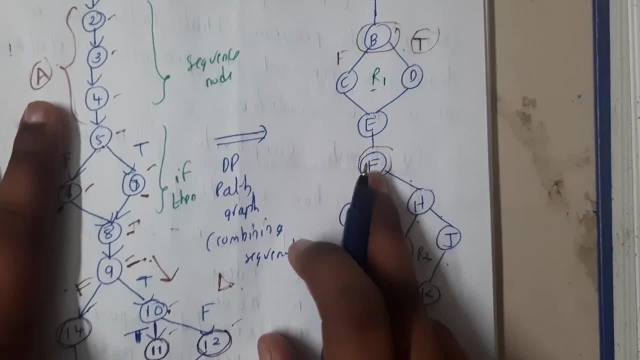 going in this way. so this node says about whether it is a triangle or not. so, based on this output, only this node exists, guys. so here, if you get true, you can enter into this path. if you get false, you cannot enter into this path, guys. so that is the reason why i assumed that you can go in that path. 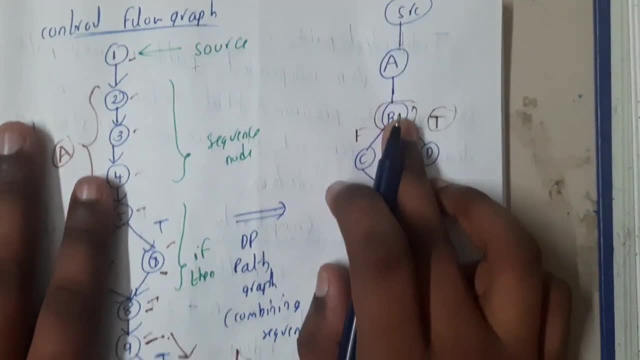 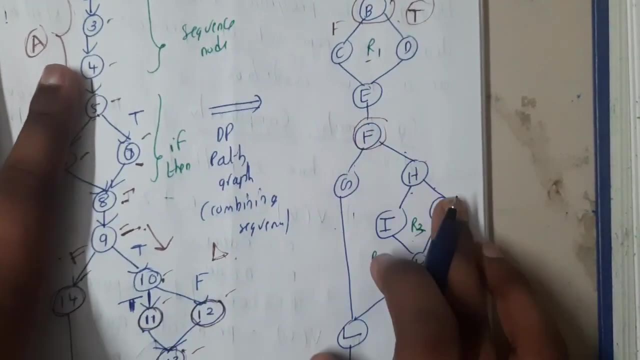 so i gave in that way. okay. so you'll be starting here and if it is true, you'll be going through all the possibilities. okay, similarly to the second path and similarly to the third path, whereas if it is false, you'll be directly moving on to the left side only. so in this way we will. 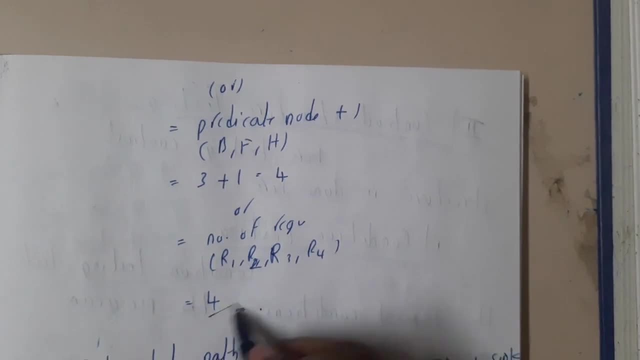 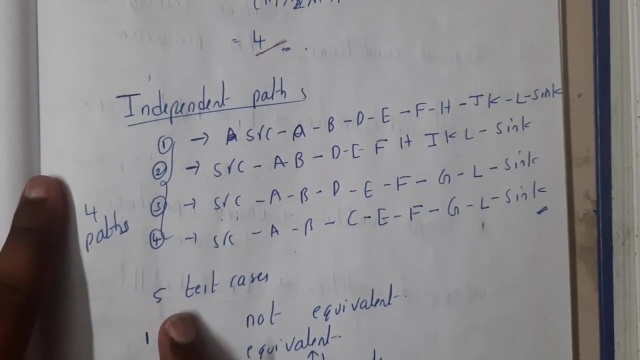 we will be checking the multiple paths, guys. so, based on your result, by applying formulas, that many cases, that many independence paths, only you'll be getting okay, okay. so so from these things, we can write five different or four different test cases. guys, we can write only four. 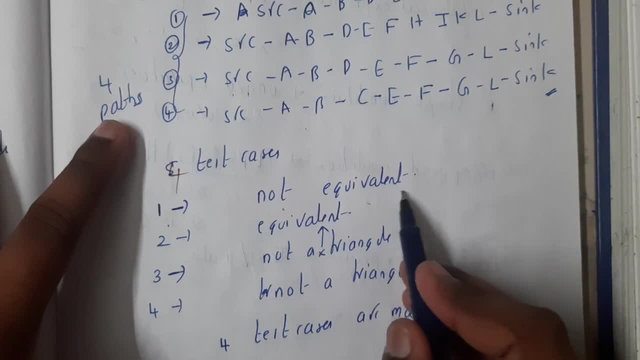 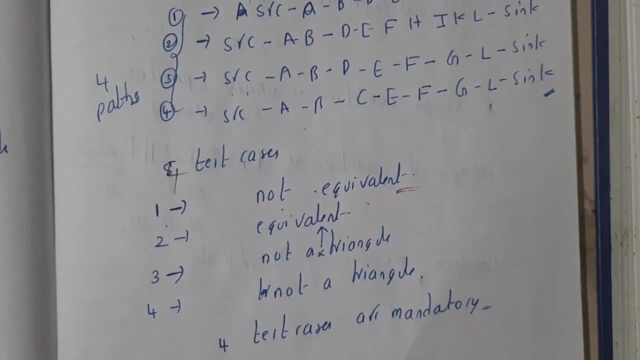 okay, so the first test case is nothing but for not equivalent. so are not equilateral triangle guys. i i multiple times i wrote equivalent, equivalent. sorry for that. okay, so the second statement could be for equilateral triangles and the third statement is nothing for not an equilateral triangle, that's. 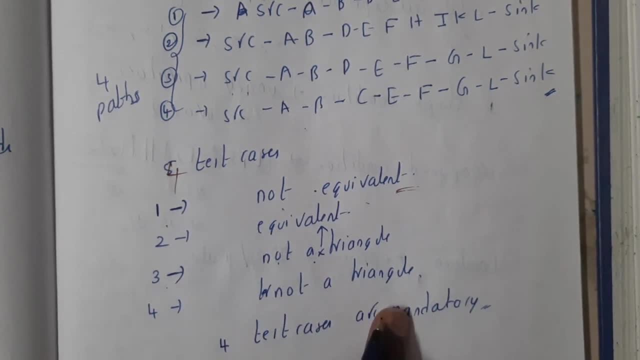 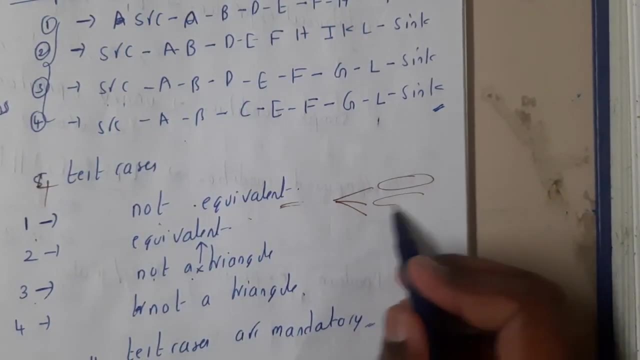 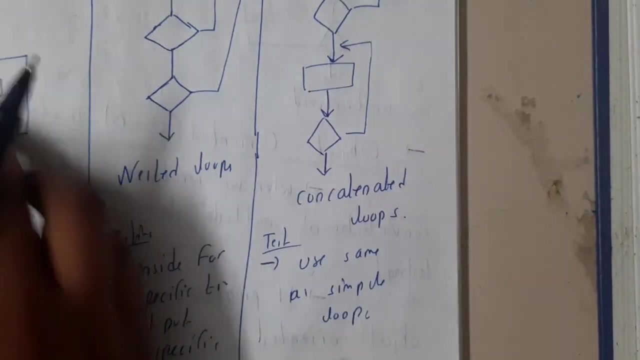 nothing but not a triangle. and the fourth statement is: nothing but not a triangle. fine, okay, so these are the four mandatory cases, or you can even manage in three different cases, also, like not equilateral, equilateral and not a triangle, because the triangle is only divided into these two, right, okay, so that's the quite simple method. okay, so i hope everyone got a. 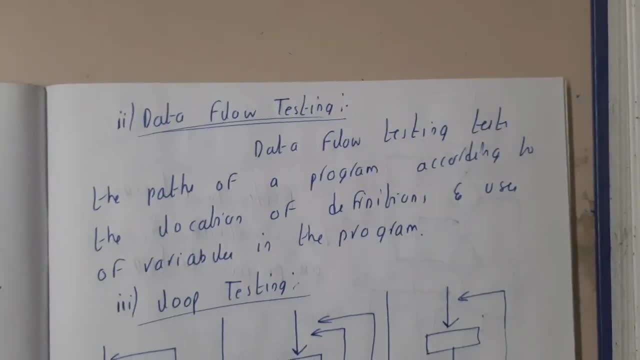 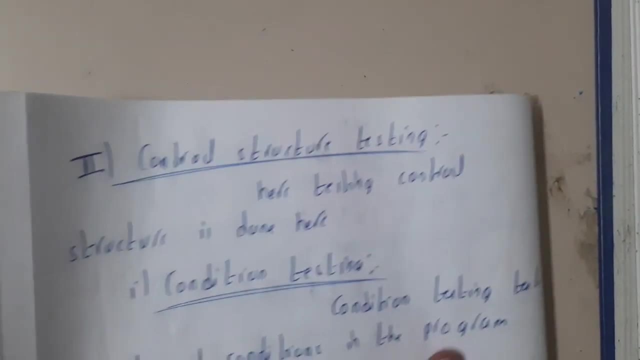 small idea on this, so i think already the video has been became a bit lengthy. okay, better, let us complete it, guys, because you will be done with one of the most important topic, right? okay, let it go to 17 or 18 minutes also, it's fine. okay, so let's give me two to three minutes. i'll be. 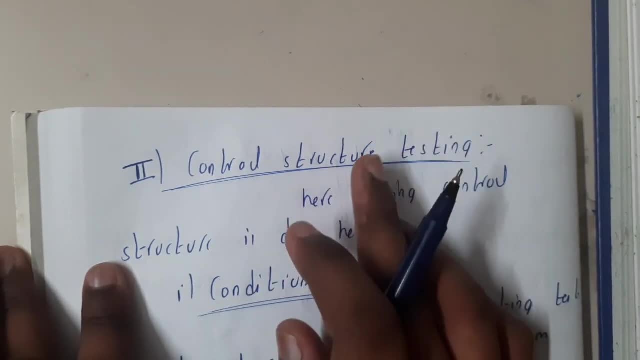 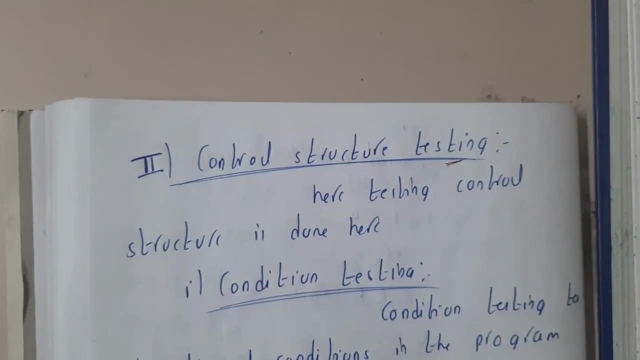 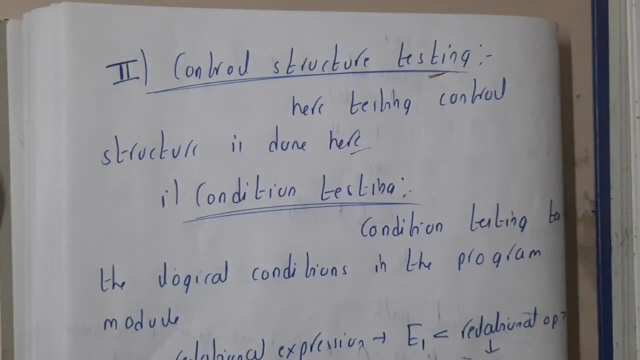 completing it, guys, don't worry okay. so now the second type of method which they will be approaching: in white box testing is nothing but control structure testing. so here you will be drawing the structures, guys. okay, so here testing control structures is done here. okay, so conditional testing is nothing but conditional testing. tests the logical condition. 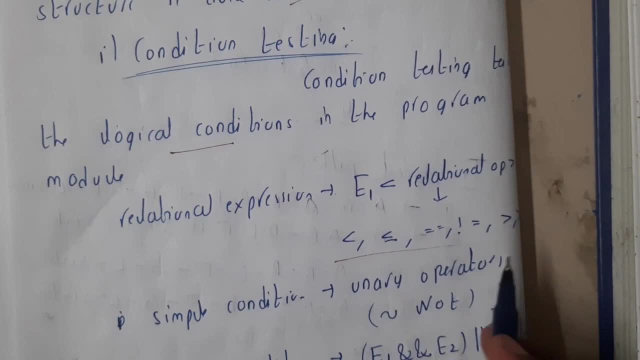 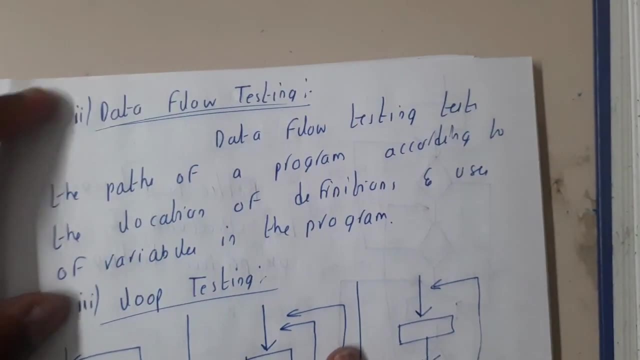 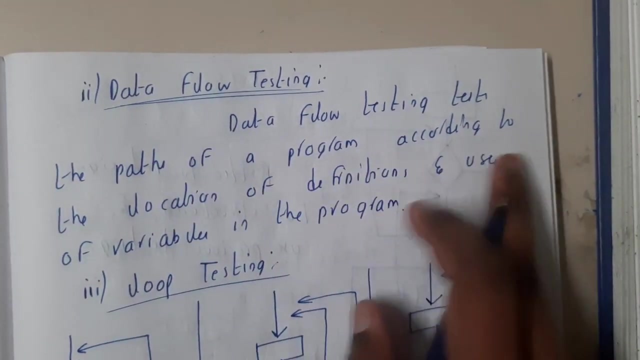 in the program, like the relations, like less than greater than equal to, with not operations, and operations true or false with boolean, okay, so you'll be checking those things and the next will be data flow guys. so how data is flowing. so data flow testing tests the path of the program according. 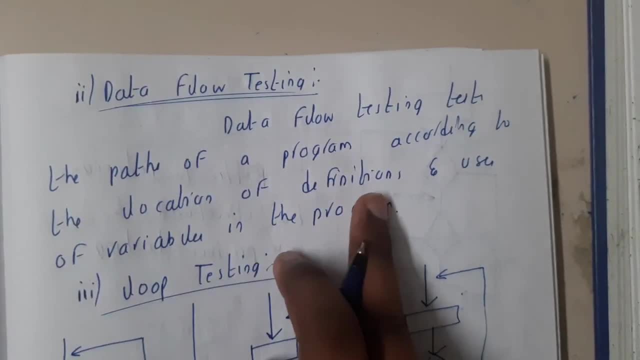 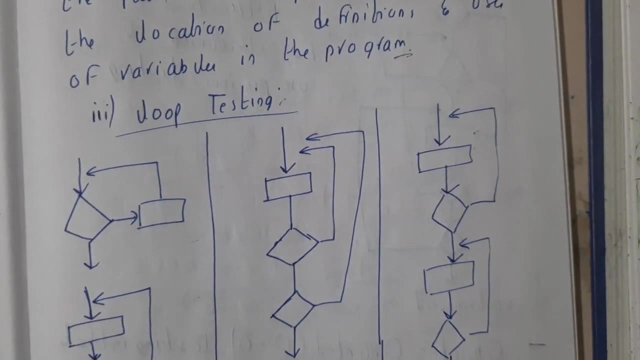 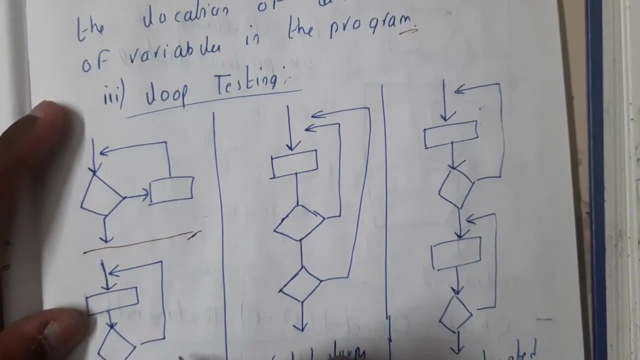 to the location, guys, okay- of the definitions and uses the variables in the program- okay. similarly, we will be having loop testing. so basically, depending on the loops also, we will be considering some test cases. so if you observe here, so this is a simple loop or this is also a simple loop, right? so here this is. 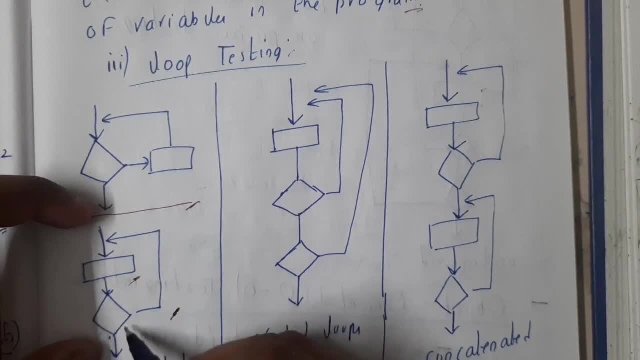 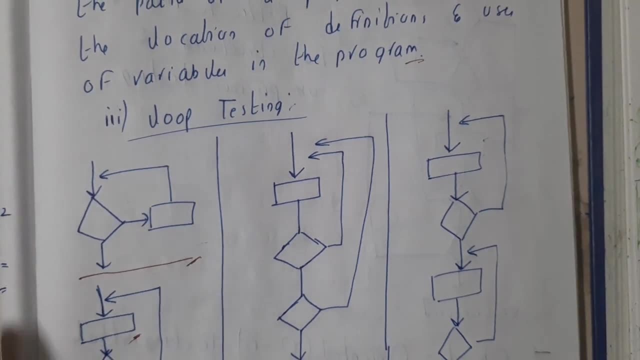 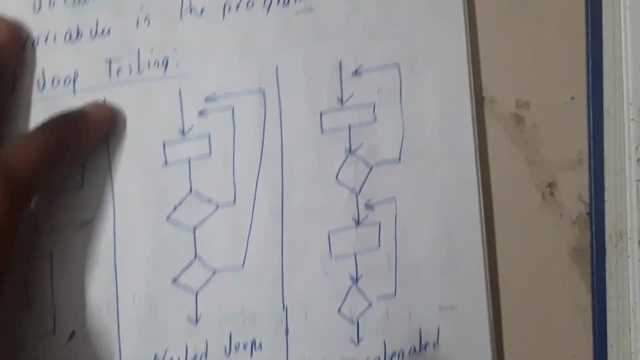 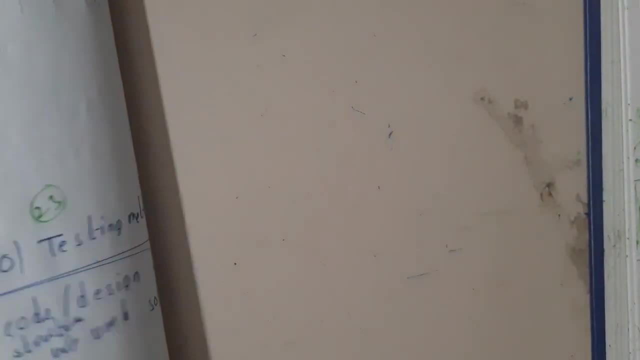 we are having here concatenated loops, so one after the other, okay, and here we are having a mixed loop which is a mixture of everything, so there is no particular format, okay, so if you observe here- so we wrote the testing- also what is required? so the first thing you should check: 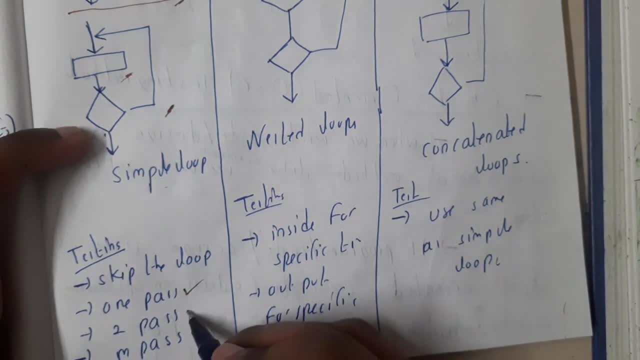 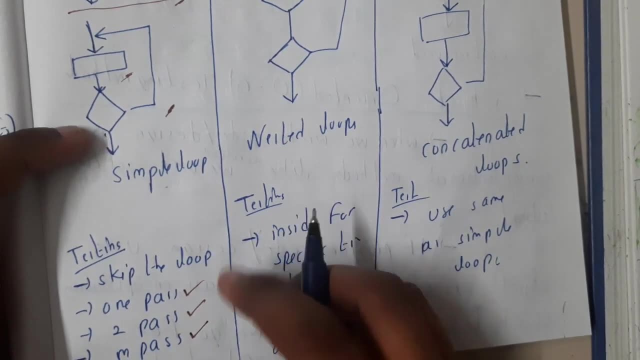 is nothing, but you should pass it for one time and you should pass to pass and you should pass and m pass. so particularly, you should pass for once, twice and you should pass for some minimum number of times and in one chance you should need to check the skipping whether it is skipping or. 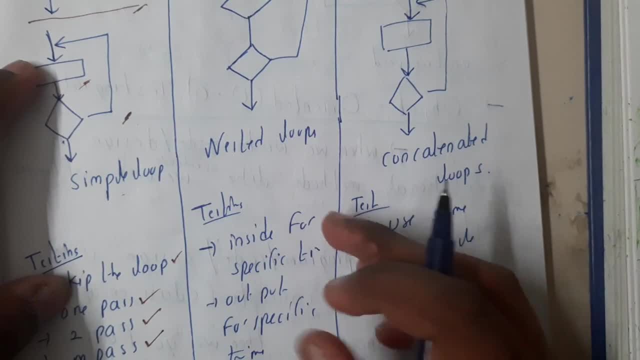 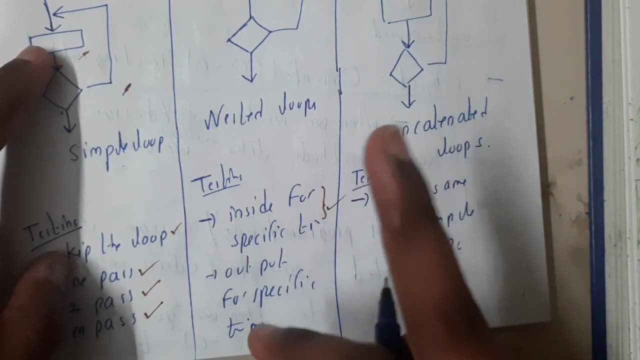 not okay. so in the next, for a nested, you will be checking whether the inside function is working properly and it indirectly depends on the exterior and interior functions are both dependent, right, so you should check those dependencies based on the outputs. so basically, for one after the other. 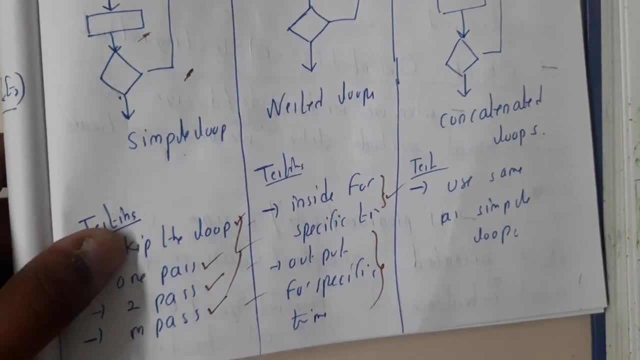 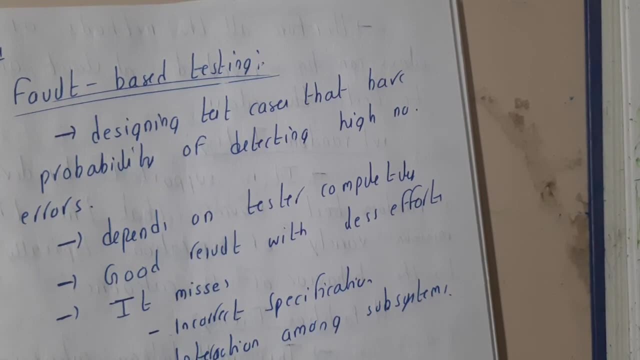 also we'll be checking the same thing, skipping the loops one pass, two pass and m pass, okay. so i hope everyone got it some basic idea or clear idea about white box testing or glass testing. so in the next lecture we will be going through some basics about object oriented testing methods. okay, so let us meet in the next lecture, thank you, thanks for watching.